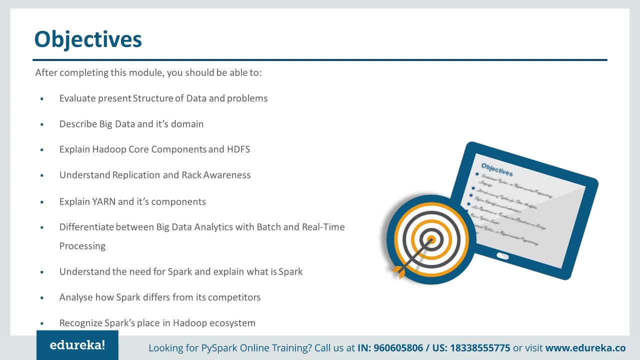 to explain What are some of the core components in Hadoop and what is H2O Fs and its role in the Hadoop ecosystem. We will understand how does replication and rack awareness work in a big data appliance. What is yarn and some of the components and what is the? 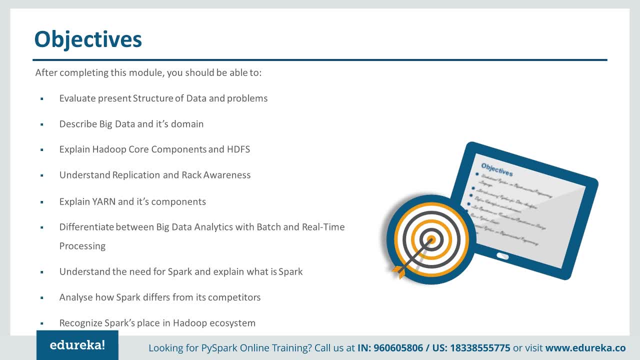 significance of me and where does it actually fit in. We will also differentiate between big data analytics with respect to batch and real-time processing. And, finally, we dive into the purpose of this course: understand the needs of big data analytics. And finally, what is the need for a spark, explain what it is and analyze? 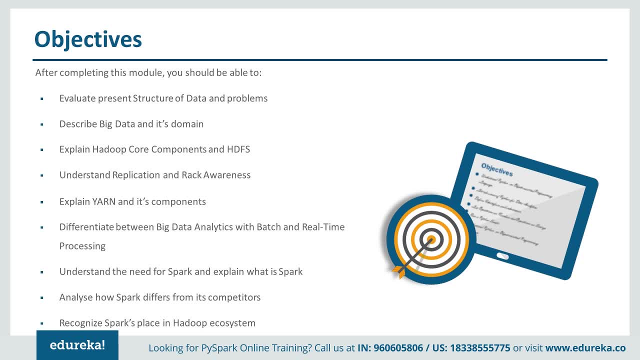 how does it differ from its competitors? And, finally, what is its space in the Hadoop ecosystem? Where does it actually fit in the Hadoop ecosystem? So, as you would notice, some of this- or I would say most of this- is theoretical in module first. 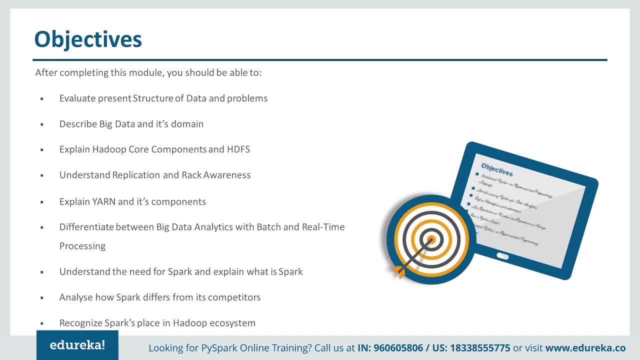 but module second onwards, we have all hands on again until module 6, because module 7 will be slightly theoretical or mostly theoretical on machine learning, and followed by that again We have all hands on until module 12.. So we'll start with Python basics. 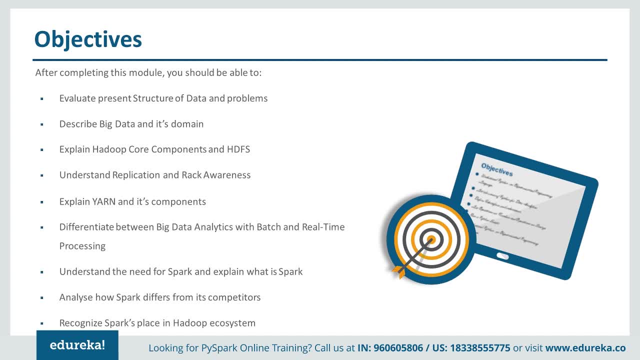 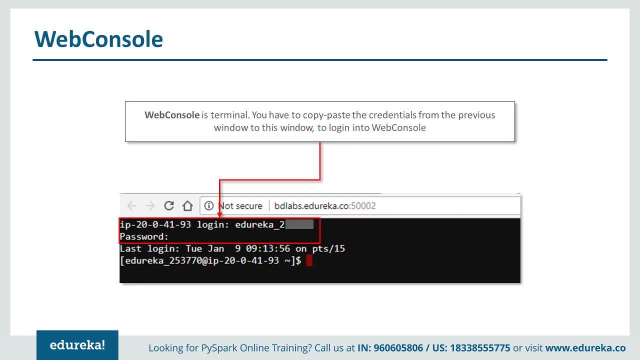 Even if you don't know Python, so that should be helpful for you, and then, followed by that, how to use Python in a big data context. All right, let's dive in. So we have already covered cloud lab access. in case you want to try out any one of these, 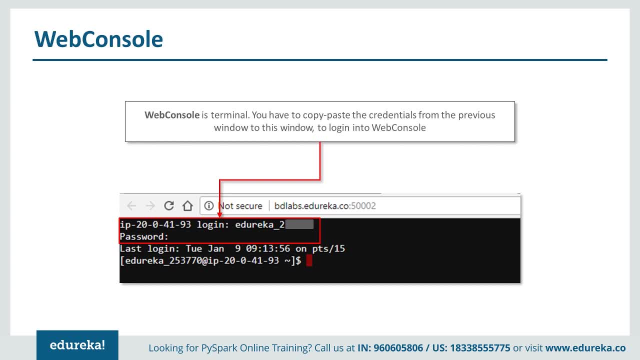 to make sure you are able to connect. So web console is the terminal. you have to copy paste the credentials from previous window to this window to log into web console. That essentially means hit on web console. that will open up in a new tab. You may copy your username. paste it here. control V- enter. 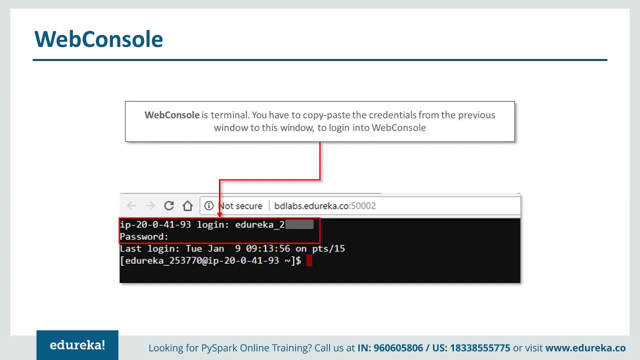 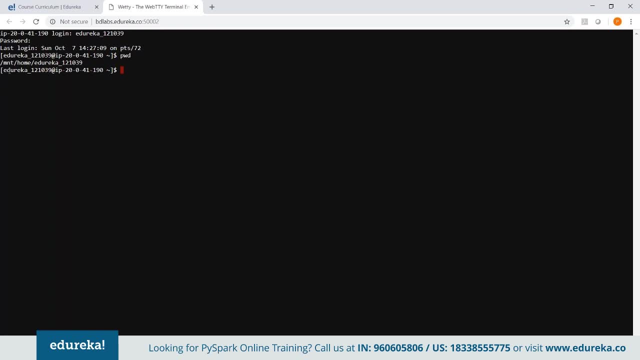 and you may copy your password. copy control V, enter and you are in check, your present working directory. So each and every one of us, the directories are organized with our user ID as the last point in the directory. Everything will have Mount home as the prefix. 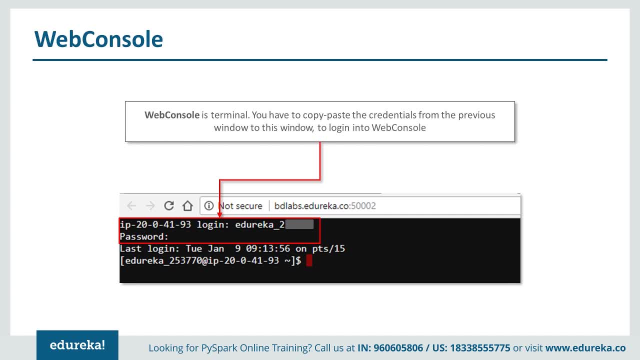 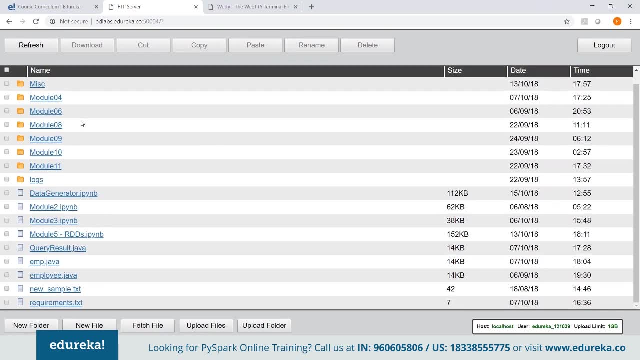 and if you try to connect to this using FTP, it already has my credentials. That's good, but you may enter yours. So it takes me to this point where it shows all this: files and folders, right, But if I go to web console- or did I close that? 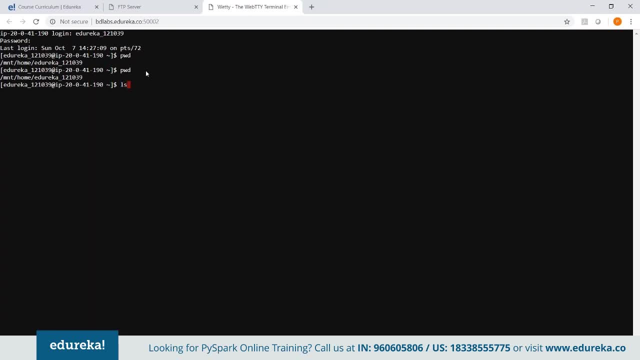 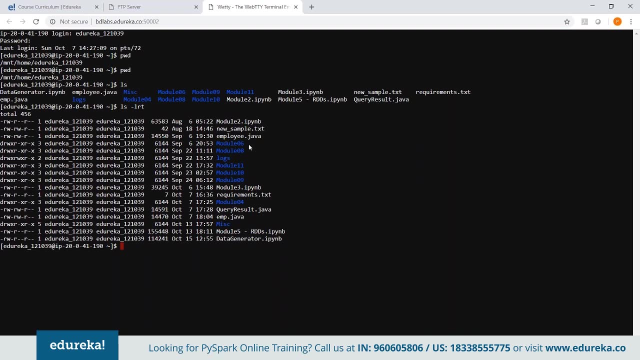 So if I check present working directory and I say LS, or rather less alert, I see the same information here. You could see module 4, 6, 8, 9, 10, 11 as the directories. and then we have a bunch of files like module 2, new sample. 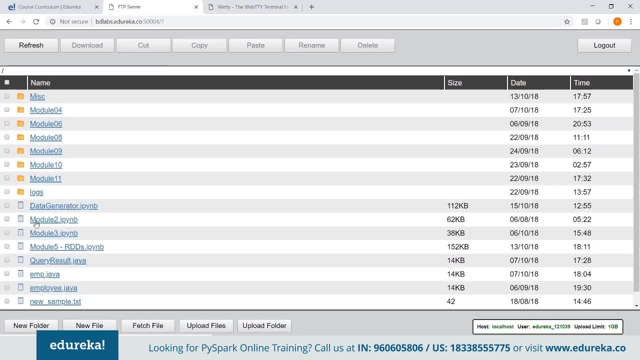 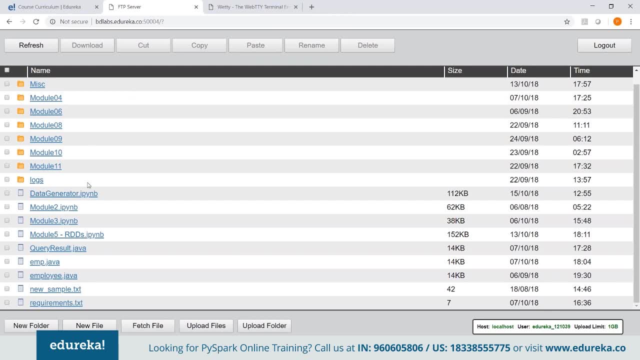 employee Java right. You would see the same content here. So FTP is a tool that helps you connect to the terminal in the using a user interface, and it gives you these options: You can refresh it, You can choose something and you can download a folder. 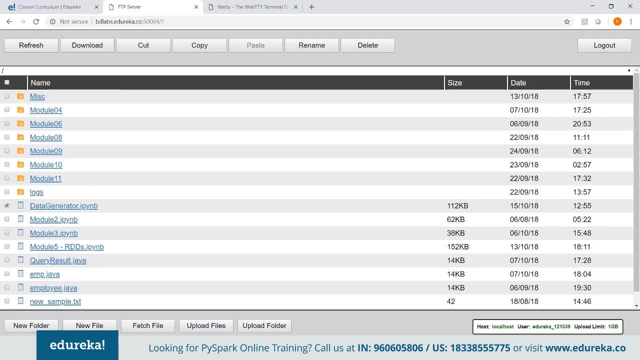 You could download a file. Just select the file and you will download it. So I think this also answers one of the questions we had with respect to downloading content- and you may also upload files to it. So you may choose a file, like, say, upload file. 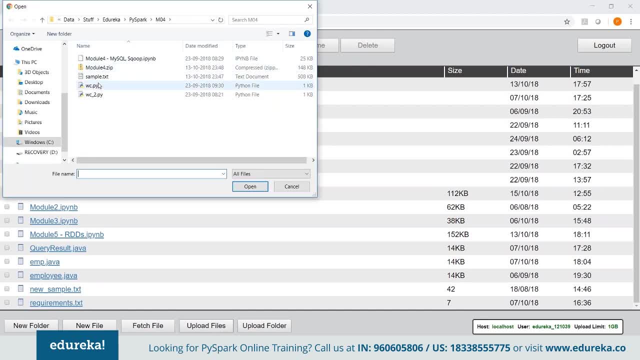 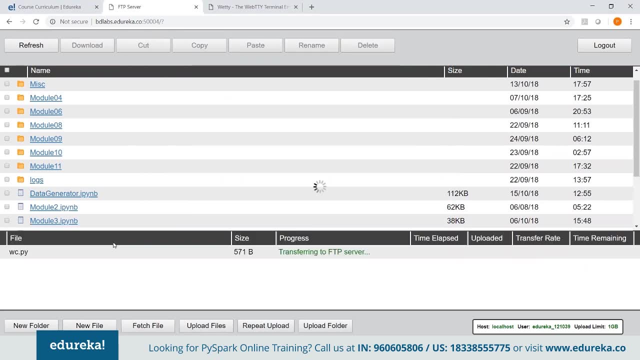 It takes me to a particular point wherein I can choose something. Let's say word count dot five. That's not there. I don't see it. word count dot pi open and I could see that uploaded on 2010.. That's today. 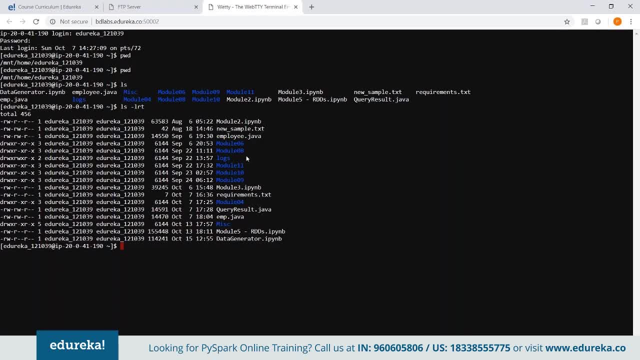 I can delete this. So this is our interaction in the form of a user interface and that lets you connect to your local system to upload or download anything, and you can also organize content directly on the terminal, moving files from one folder to another or renaming files. 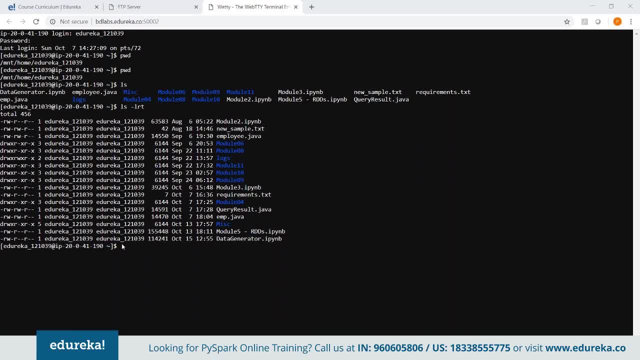 renaming folders. So this is a Linux environment. So if you are not familiar with Linux, you can Google some of the basic commands like copy, move. But if you even don't want to do that, all the content that I'm going to share with you. 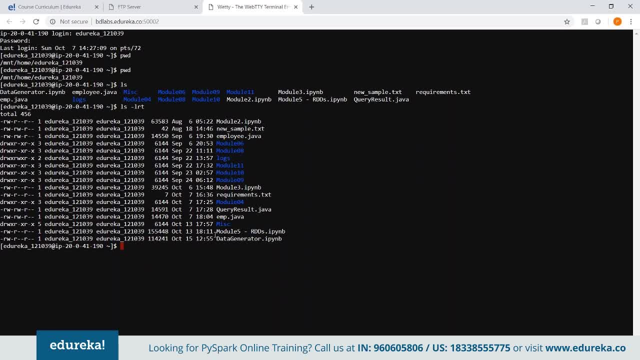 It's going to be organized in the form of these modules so you can unzip that on your system in the form of a folder that will give you module 0, 6, module 0- it as the folder names, and then directly upload the folder. So you'll essentially have a similar kind of content. 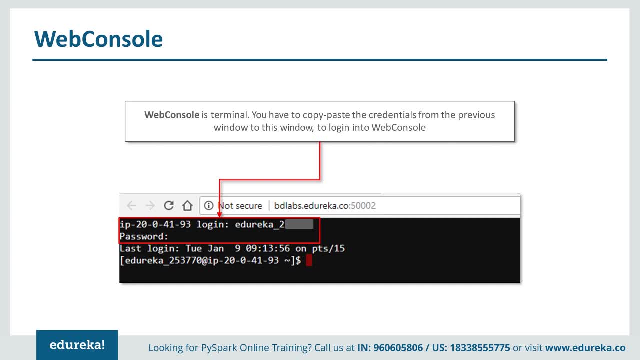 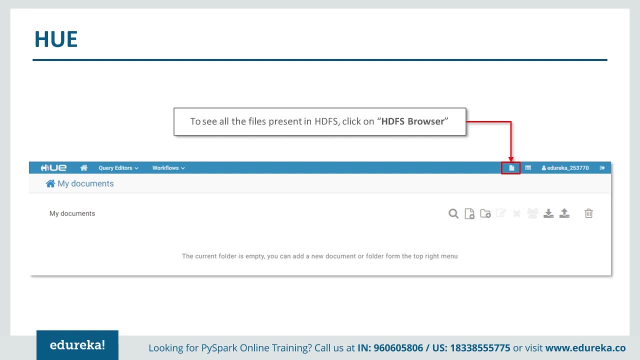 under your user ID. So, coming back to content, that's how you access web console. Now here is a browser to access HDFS. HDFS stands for Hadoop distributed file system. Like we have a file system on our operating system, Hadoop has its own file system. 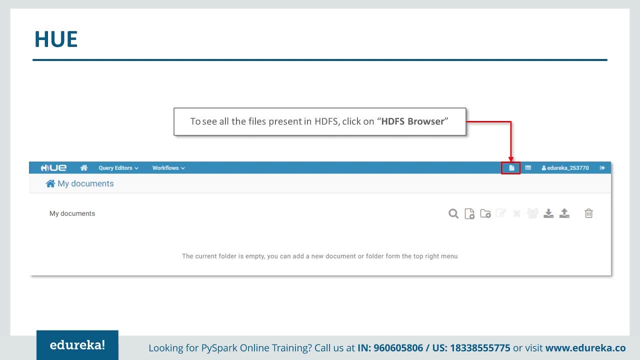 and that means the files are stored in a certain way, I mean they are not accessible to naked eyes unless you use Hadoop commands to access those files or look at contents within those files. So here's a tool that simplifies much of those tasks, saving 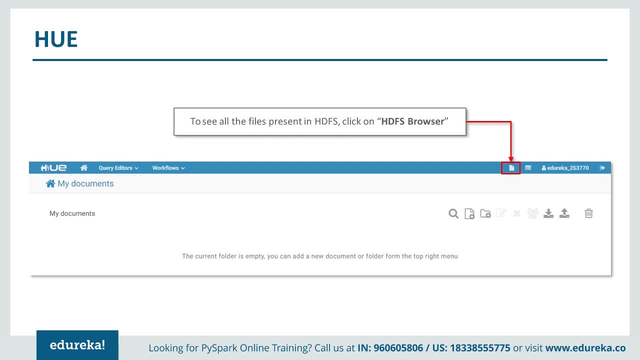 you the effort of writing HDFS commands and you can directly look at files. upload files to HDFS. download files from HDFS: right, So similar to an FTP file that lets you connect to cloud you let's you connect to HDFS under your cloud account. 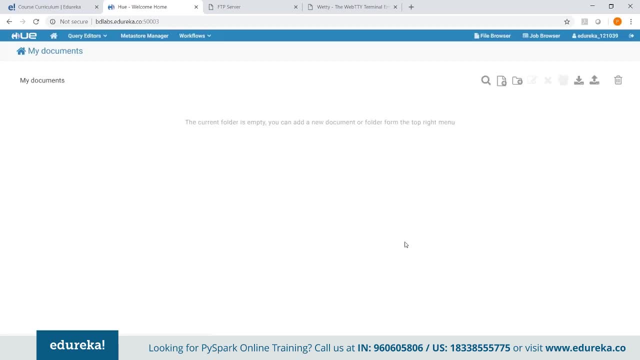 So let's open a you. I have saved my credentials on previous sessions, So I do see that directly. this takes you to the home page, My documents. that often shows up as empty, but if you hit file browser you will see most of your content here. 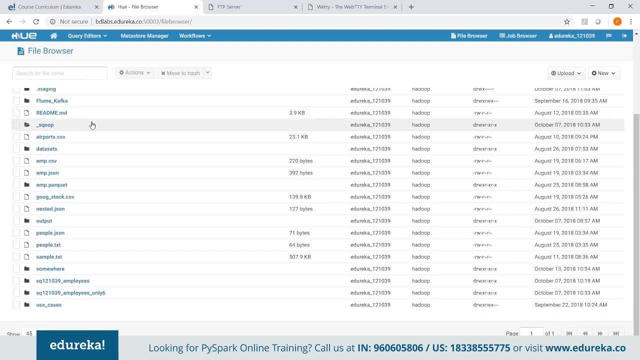 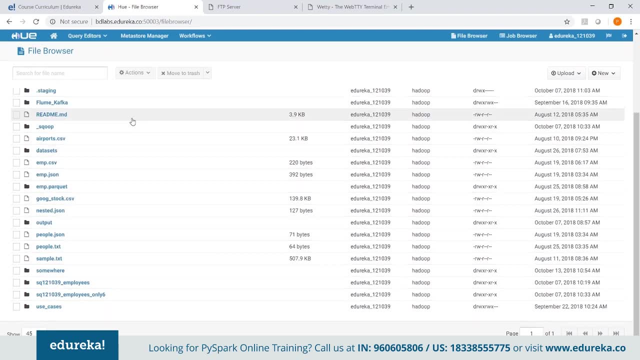 So this is where we are going to save some of the files for upcoming hands-on, like data sets, airport CSV, employee, All of these. These are going to be referred in some of the upcoming modules and we can choose any. we can say delete this directory. 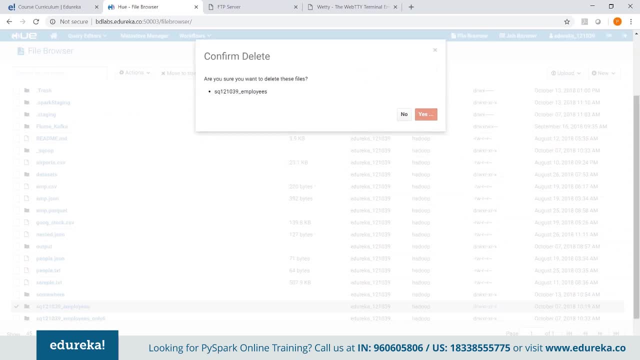 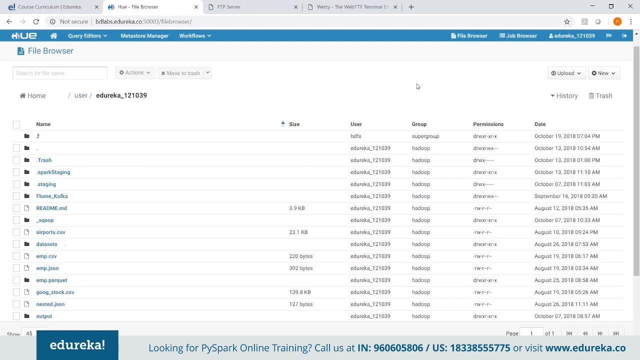 So move to trash and get a prompt: Yes or no delete. and the directory got deleted from HDFS. So much of this will be clear when we cover HDFS, and I will show you how to see a list of all these using Hadoop commands. 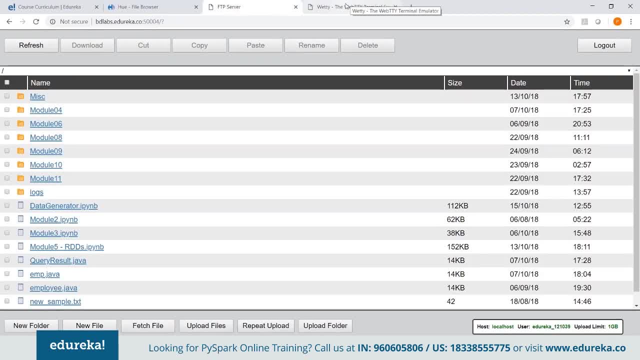 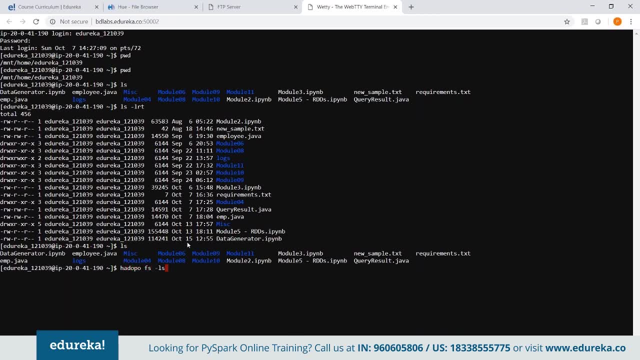 We cannot see that using regular file listing commands on Linux operating. So if I do this here, I don't see it. But if I say Hadoop FS LS, it shows up the exact set of files that we see there right airport CSV data set. 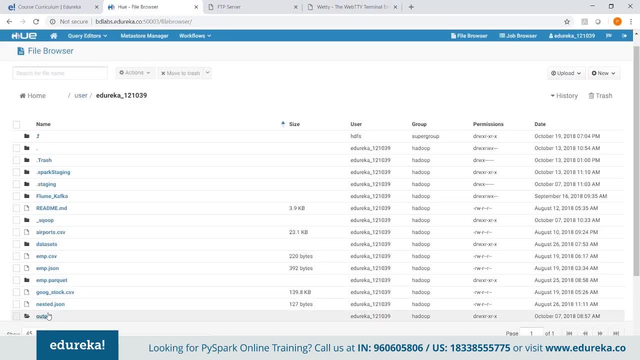 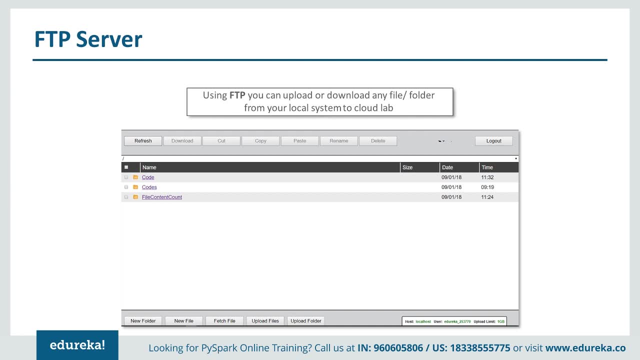 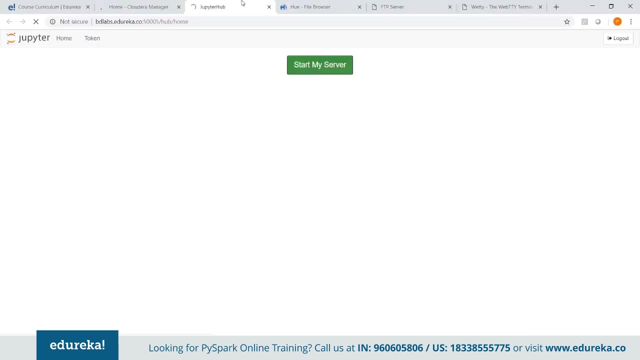 employee CSV. we see all these files there. so much of this is clear when we touch upon HDFS commands and then FTP server. We have already looked at coming to Jupiter notebook and launch that in a while. Then we have cloud era manager. So when you log into Jupiter, 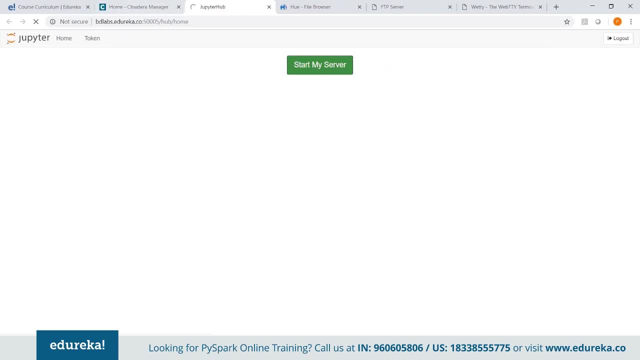 this is the first thing you'll encounter. start my server. It did not prompt me for my credentials because I'm already signed in, But when you do it for the first time- or probably several other times as well, If you are signed out you will be required to enter your user ID. 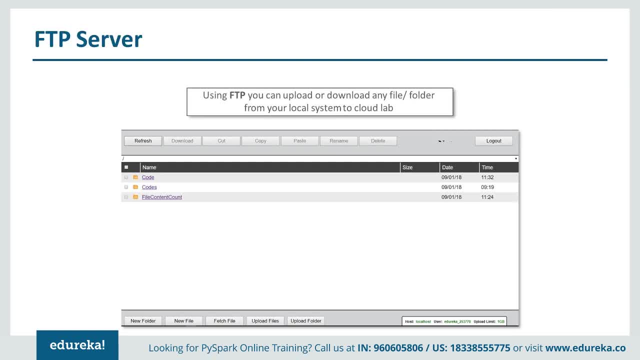 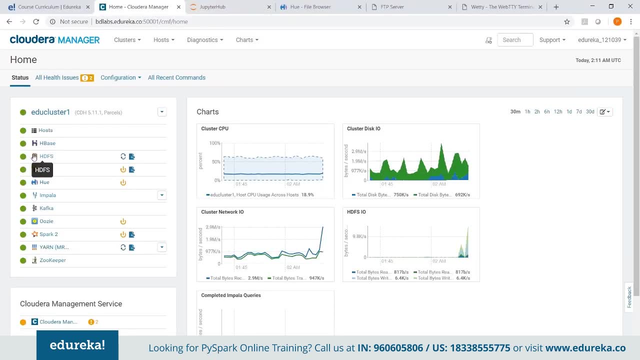 and password for each of these portals. We do have the same set of credentials, So you don't have to keep a track on what should be used to sign into cloud or a manager, or to Jupiter. So in cloud era manager, it talks about the cluster. 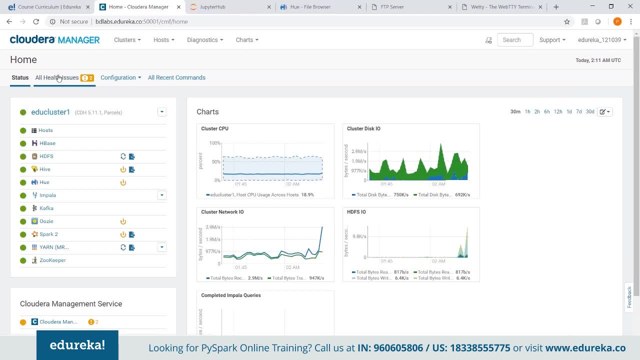 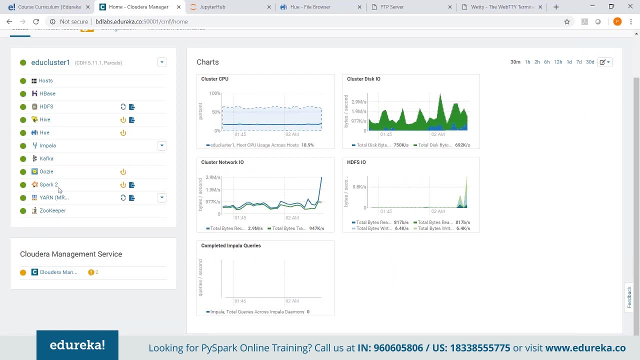 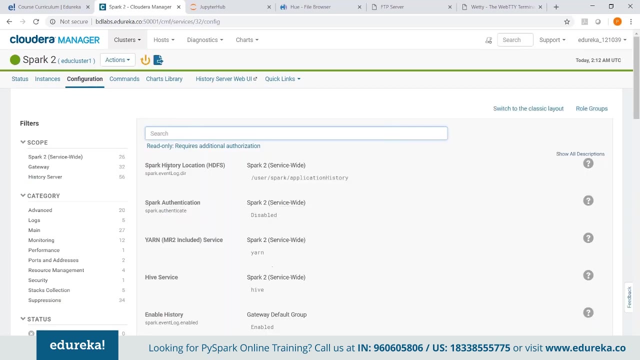 We call that as edu cluster one. There are certain health issues, but probably not related to the components that we are going to hit in initial set of modules. So we should be good. This has a spark cluster configuration details You can look at. the configuration set tells you. 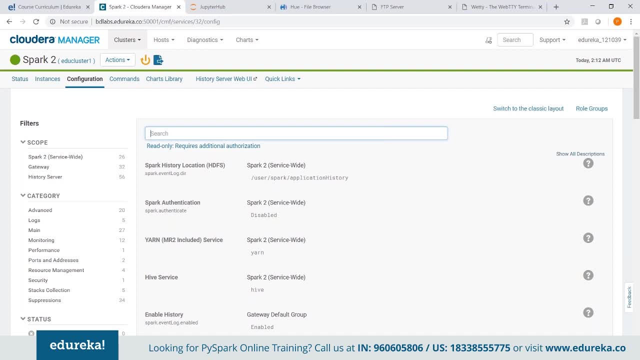 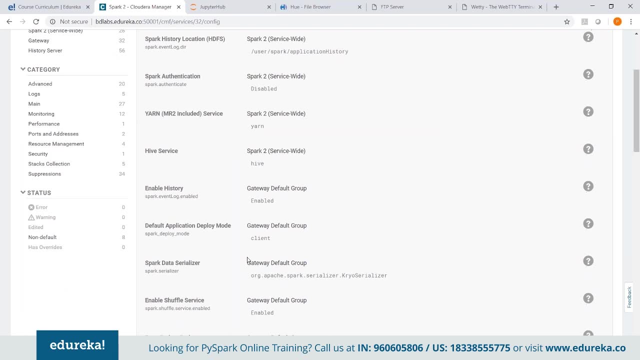 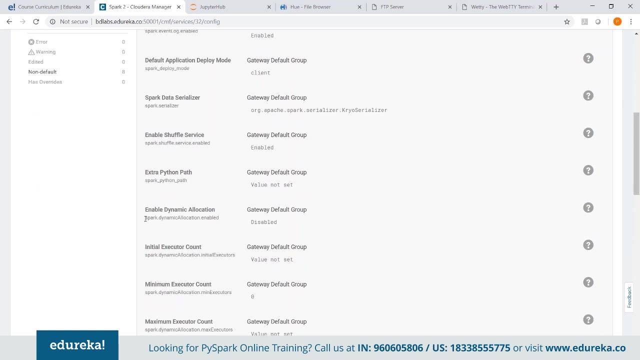 where is the application directory, and it also tells you what is the corresponding spark property that has been pointed to this particular. So essentially it's a combination of all spark properties and their respective values. We will touch upon some of these, especially like spark dynamic allocation enabled. 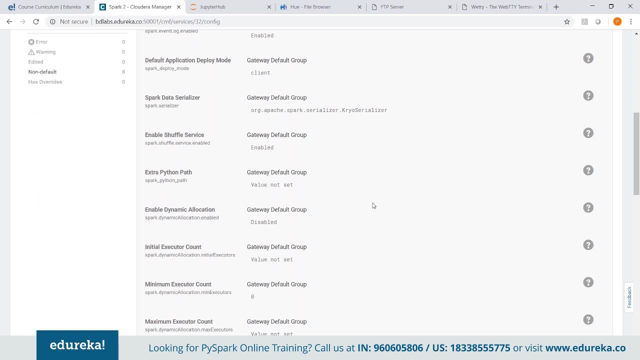 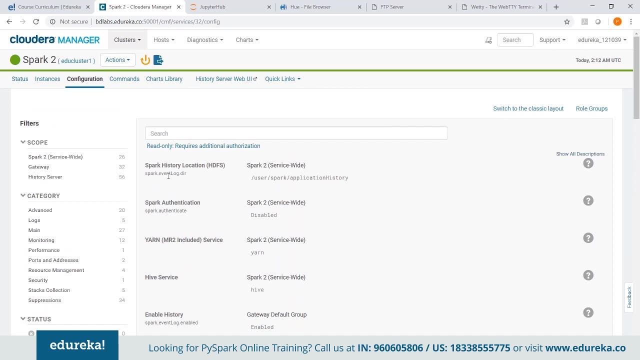 and we will enable this in few of the jobs. So usually when the cluster is set up, the admins ensure that they have some restrictive policies in place so that anyone is not able to misuse the cluster at the cost of affecting others. but then some of these are flexible enough. 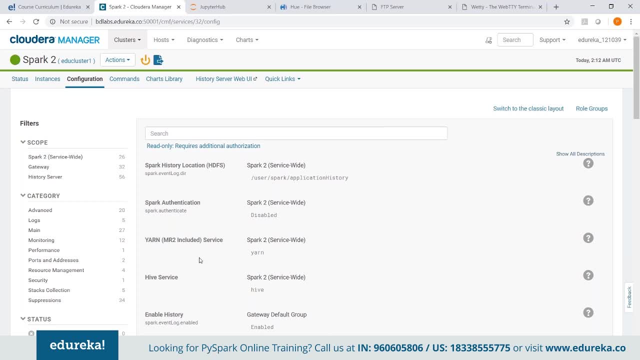 to be overwritten in one specific job. This is very helpful. So at cluster level we do have some restrictions, but when we run a job on a cluster we do have the flexibility to define something the other way to make our jobs run in a better way. 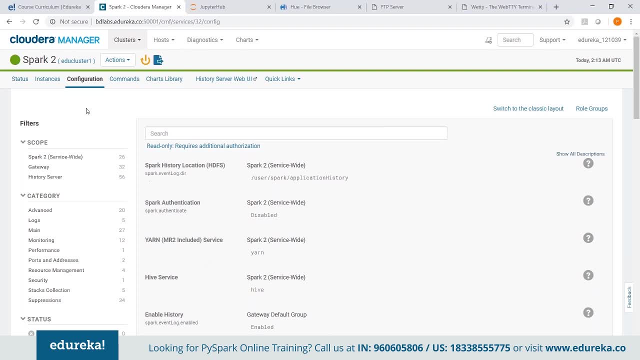 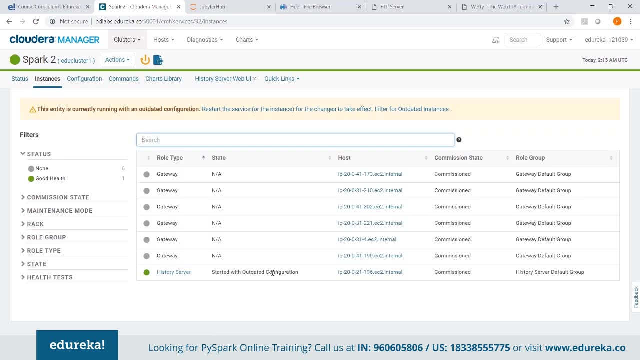 So we will overwrite some of these properties and that's where we will revisit some of these configurations. And if you want to look at the number of instances, it tells us there is a history server that's in good health. What is the state of commissioning? 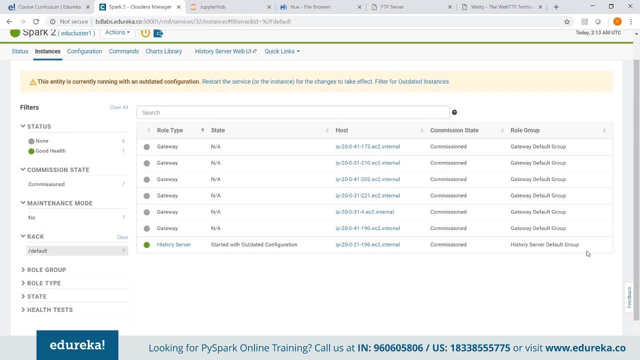 What track is being used? default track with seven nodes and there are six that serve this role as Gateway. So each of these will be an internal node in the cluster and one is the default history server that is used to track our jobs. So much of this will be clear. 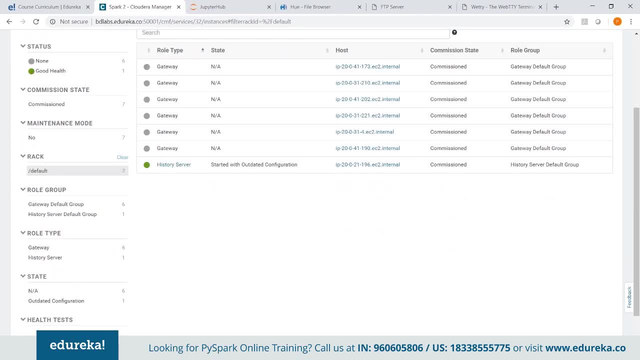 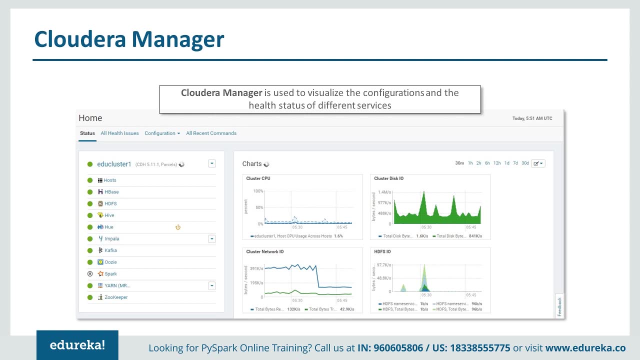 when we touch upon a spark concepts and see how to look at the status of a job. So, now that we have touched upon all the related components, we are not going into details of each one of these at the moment, but there will be times. 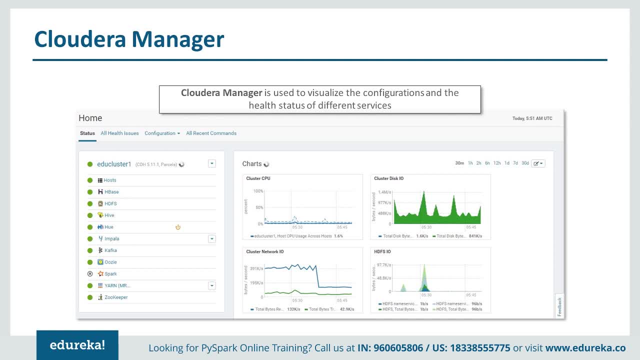 wherein we will spend more time on Cloudera manager. We will spend more time on the cloud, on a spark console, to understand the properties of a job and the details on how it is performing. So let's hold on until then, and now we will begin with the structure of data today. 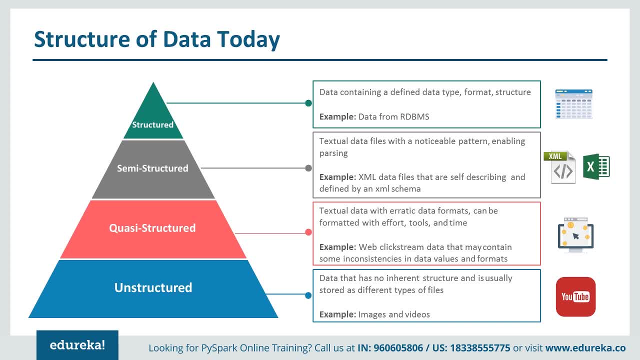 So in the initial years and as I also mentioned, as part of my experience, I was initially working on few rdbms tools: tuning things, tuning sequel queries and processes to make data processing smoother and ensure the reports were available to different levels of management at the scheduled time. 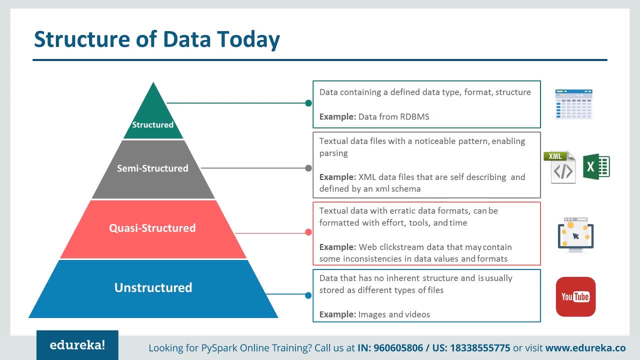 and this is something that was the case in almost every industry. You talk about ERP, You talk about banking systems or anything that had reliance on an rdbms. Few of the popular rdbms is were Oracle sequel server. later on, people started switching to open source versions of rdbms. 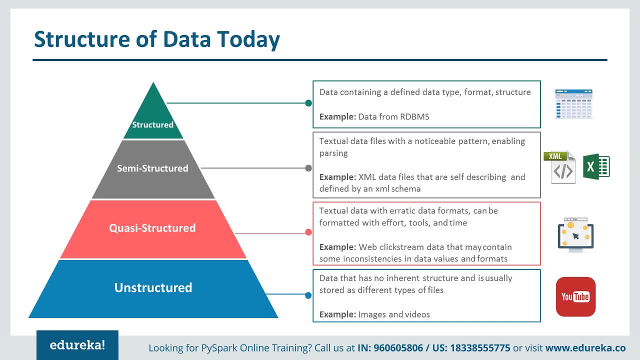 like Postgre, MySQL, and those have now become the common tools and many of the cloud environments- So Google, Amazon, they all have their managed versions of these open-source rdbms- is That you may continue to scale, or even you can have a setting enabled that scales. 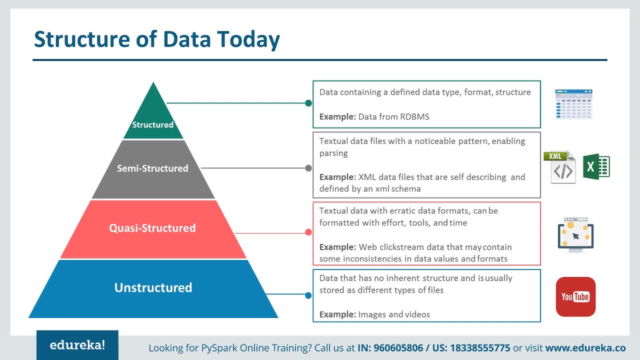 of these databases as and when you pump in more and more data into it. So the benefit with that kind of tools was they first of all required a data to be well defined in advance, wherein we say: there will be a certain number of columns, that names of the columns will be predefined, the data types. 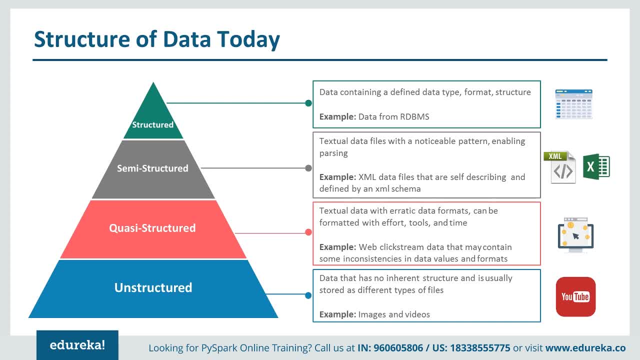 will be predefined. data will come in a format or a structure that it ideas, so that design that you would have defined at the table level. even if that did not come in that format, We will ensure that we converted to the format that fits into the table and they could be trivial issues. 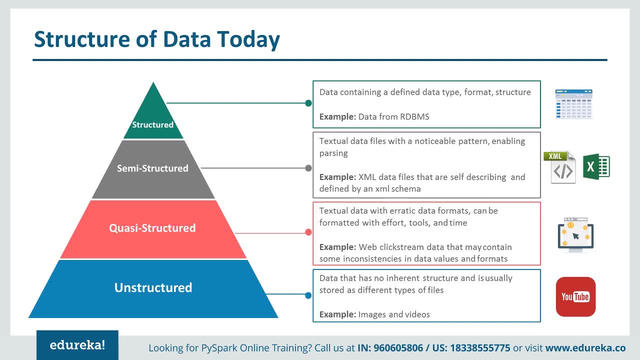 Like if you have a comma delimited format, some of the rows might have extra value, some might have less values. So those kind of issues were there in data doses as well, but it was pretty easy to deal with. followed by that We had data coming up in semi-structured forms as well. 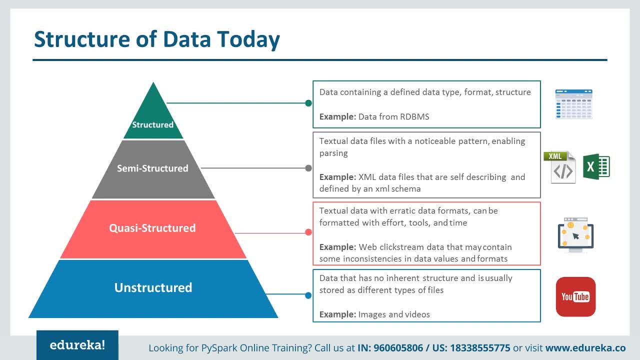 wherein we had, if you have noticed, the involvement of Java And several applications. right, and in initial days, Java's preferred mode of exchange with any appliance was to use XML and, keeping that in mind, several databases came up with their own language to parse XML, like Oracle had a library wherein you can say: use 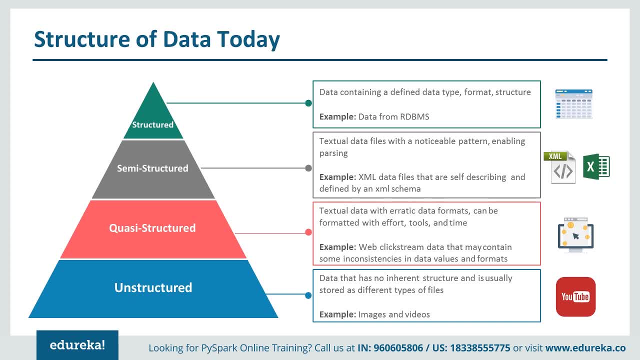 a respective connector in Oracle and say parse, similarly specifying the X paths. but that required a lot of learning, not only on XML but also on getting familiar with respective libraries and their support for XML. each and everyone had their own version, but most of the time it was easy to infer, as long 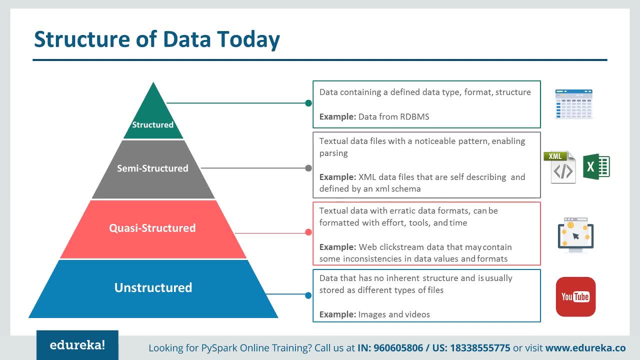 as you were pretty good in XML. but XML's were again very hard to deal with because if you think of XML in a file- right, and if the file is really huge, and if you say parse all XML, it's going to take significant time. and worst than that was organizing all XML records. 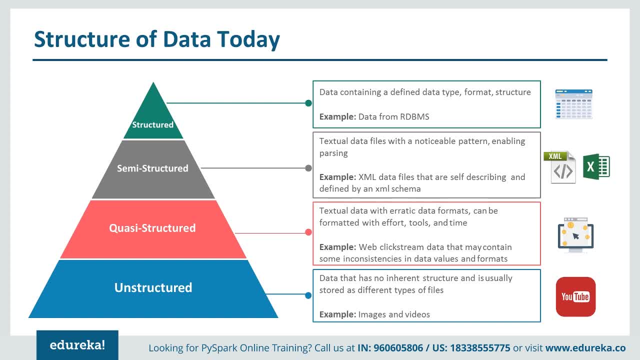 in one single line. So if it was a very verbose record like the name of the person, the age of the person, and then it let's say you have an XML node called addresses. You may have more than one address. You may have a temporary address, a permanent address, 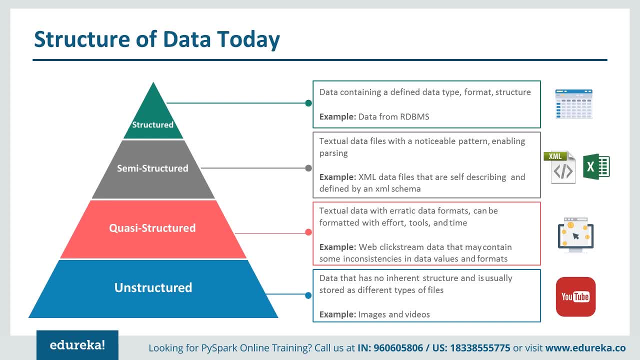 and office address- or that's the case with emails and phone numbers as well these days- right, So that will be like nested XML containing different addresses, and within addresses They could again be split fields like City, State, country and all. so dealing with that was again very difficult. 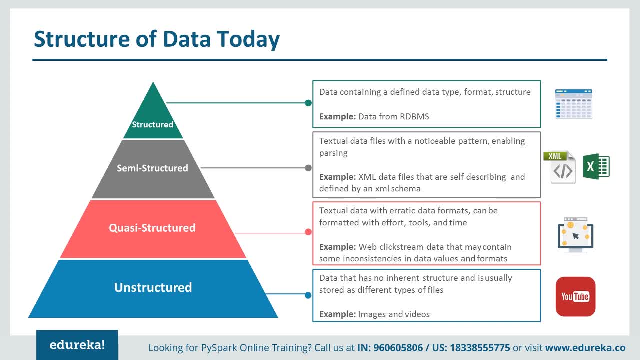 but not as difficult as they were. This is the kind of data that we see today, So we'll come to that as well in a while. So that was the second level or second era of different formats of data that we were dealing with. then came a quasi structure format, again making 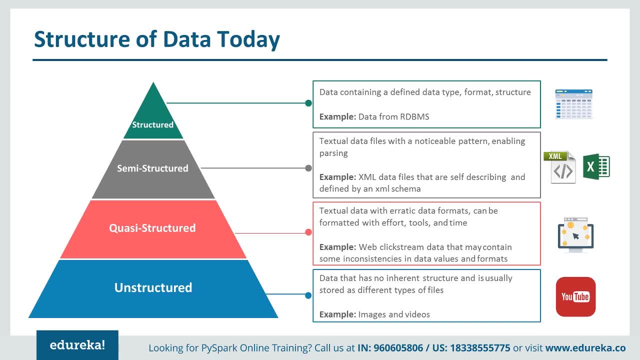 the structure more loose. So as and when the data structure started turning loose, newer tools evolved, simplified format, and that was the case with our DBMS and XML formats as well. But then in initially it was pretty hard to deal with those simple formats, because these days 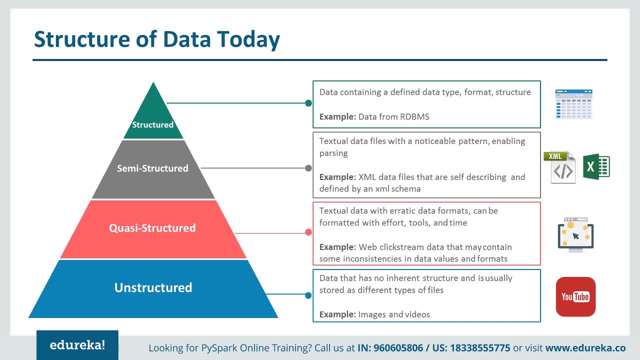 if you look at the data, it comes in all different varieties, especially if you are streaming from websites like YouTube, Twitter, Facebook. they could be post in the form of a text, image, videos, or it could be a plain file as well, like a spreadsheet, a word document. 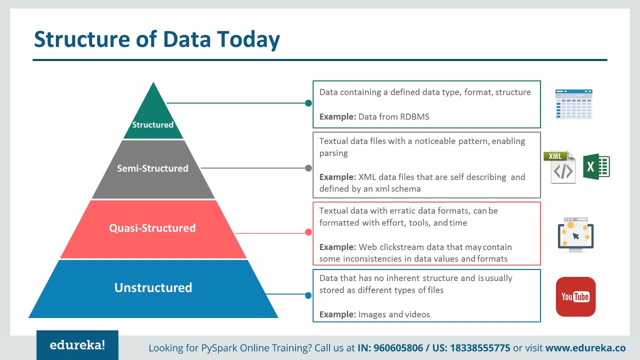 So dealing with all these formats is pretty hard, But then these days the libraries have also become more sophisticated, making our life more simple to deal with that data. So, coming to the quasi structure, We noticed that we did have textual data, but there were a lot of different data formats. 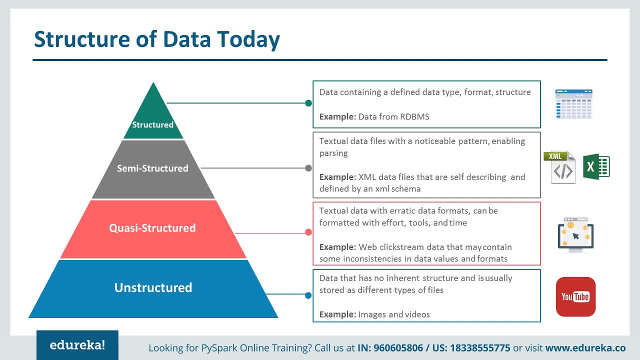 that were involved in that particular data right and it could be formatted with some effort, but it required a combination of tools, not always possible with a single tool to deal with, and time was a critical factor in dealing with that data. So an example here was web clickstream data. 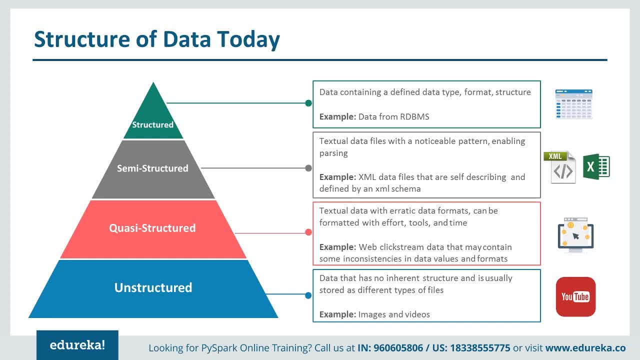 that would contain several inconsistencies in data values and formats. So if you are set up a website or if you are familiar with web development as well, right, you would know there are a lot of analytics that goes on these days around identifying those parts of the website which are least visited by the user. 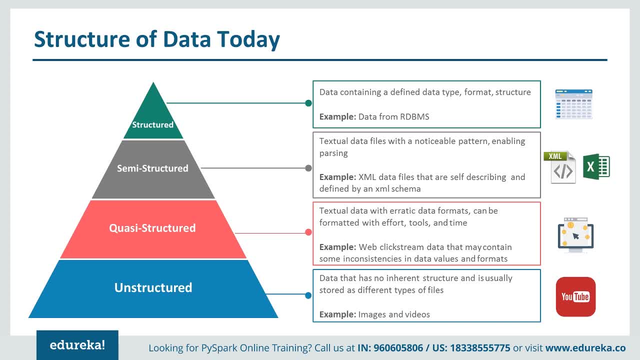 or most visited by the user, and when they are most visited, are there any errors or challenges? when they are least visited, how to improve the visibility section or the visibility of that particular section on the website, right? So all those analytics and it actually goes pretty deep. 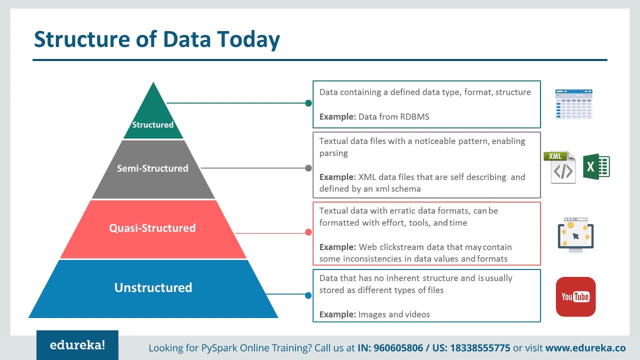 understanding some of the user behavior and the rules on organizing content on a website that go hand-in-hand. to make sure the website is interactive and informative and secure, But then the data that is gathered from these websites. they require some JavaScript libraries to take user patterns and access pattern. 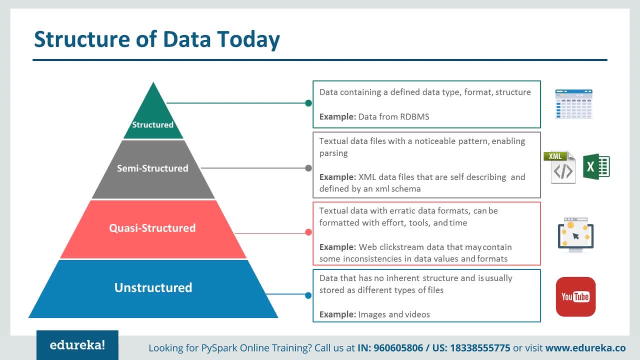 and at times there are errors, There could be network failures, There could be, I would say, crazy traffic on a website that prevents these libraries functioning in the right way. So you kind of get a broken content and dealing with that is pretty hard. But then there are libraries to help you deal. 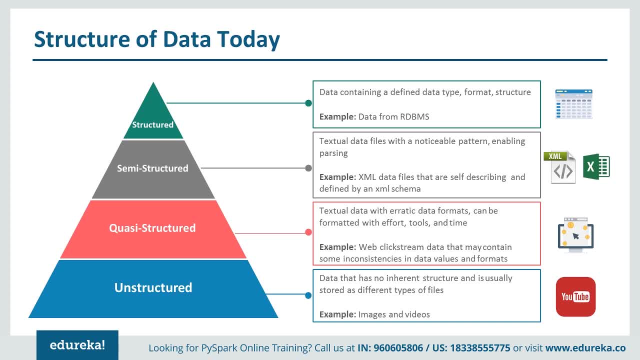 with partial content, ignoring what has not been received. I mean, you don't have a handle if something is not delivered to you in the form of data. No data, no analytics. and then came the era which we are in at the moment, where- and we do have data in different formats- 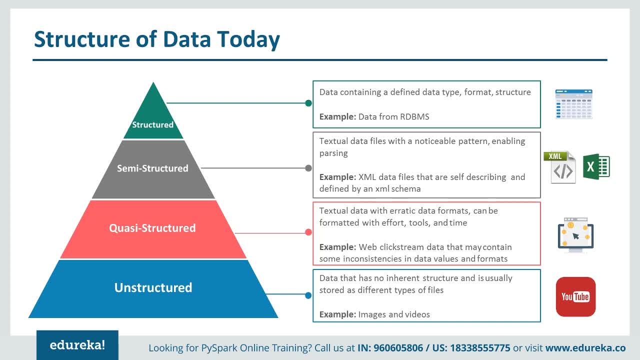 Now, I did talk about social media, right? You can also imagine what kind of data would be generated in the healthcare industry, where and when you visit hospital. you see all these kind of fancy appliances operating these days, right, different types of machines and different types of scanners making the lives. 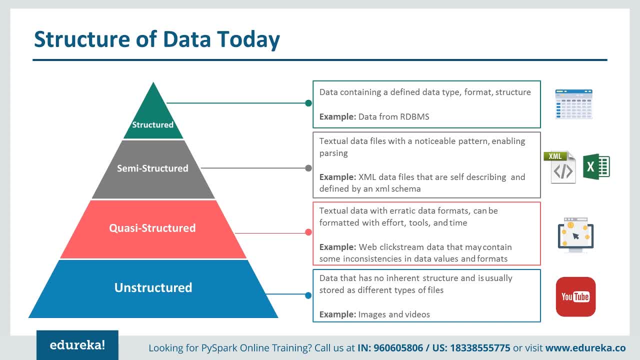 of doctor more easier and the tests have also become simple. But then, if you imagine, what kind of data would these machines be generating when your x-ray gets done? You have an image, but is that image easy to read? so that requires a different format, or the image to be saved, if you talk. 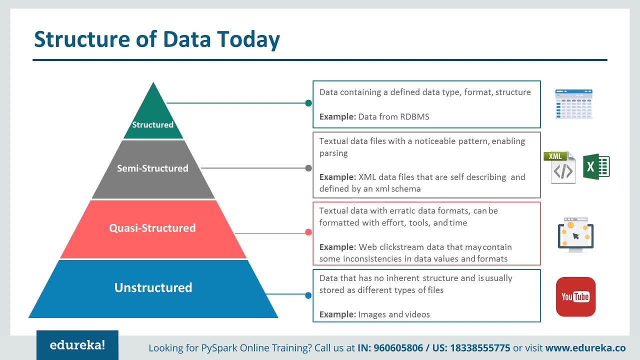 about some of the tests that that are performed these days. So they do capture a lot of a start slated to our body. Now, these starts not always go in the form of a simple text. They might be in the form of images, in the form of an audio, in the form of a video. 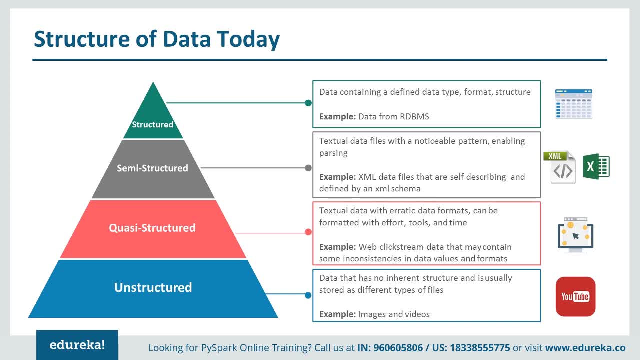 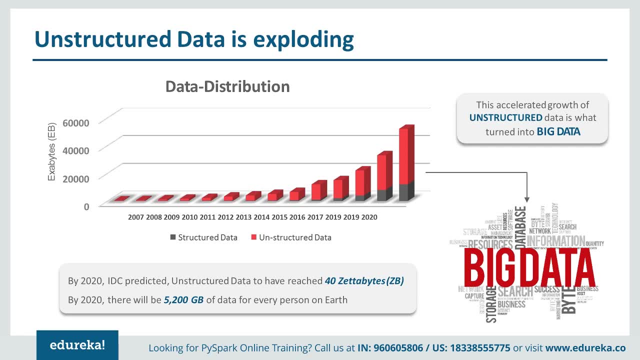 and extracting data from all these different formats is not that easy, But then, along with time and the complexity in data, there has been a significant improvement in the libraries that help us deal with these formats, and that does not mean that we do have solution to each and every format these days. 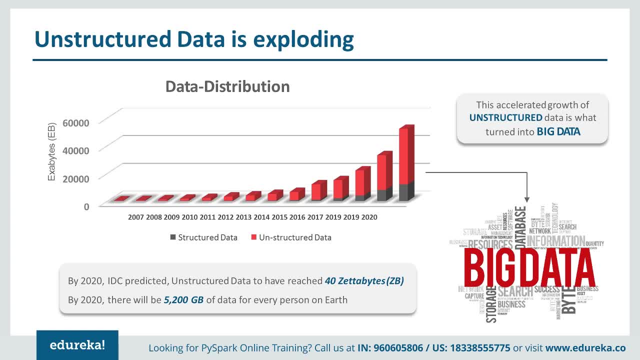 We do see newer, complex formats getting generated every day, and with the introduction of those there is a significant effort in improving libraries as well to cater to those requests. Now one good thing is, if you are new to python and if you don't know this, python already has a support. 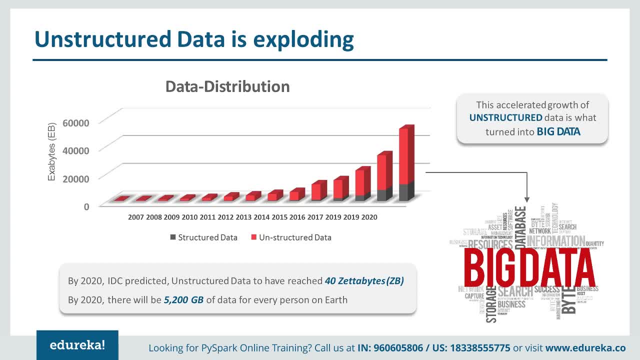 of hundred thousand plus libraries. in Indian count terms It's over 1 lakh, And if you look at any kind of a data format that you want to deal with, like some of the complex formats that I mentioned were related to the healthcare data right- 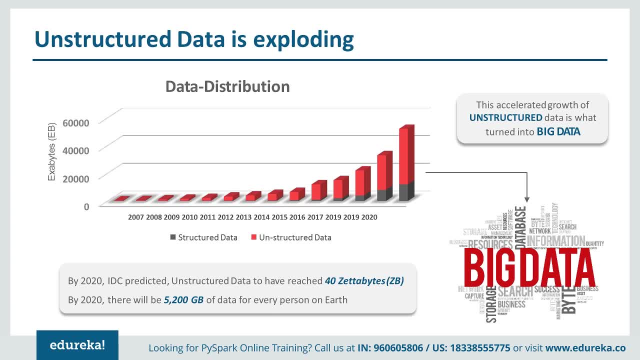 So healthcare domain also generates files that are not common to us. I don't recollect the extensions, but you may read about them or, if you happen to be on Kaggle. that is a data science competition website. If you are not a part of it, I request you to join. 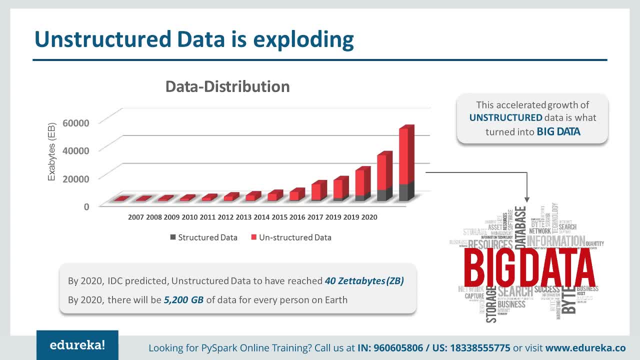 that it's a very exciting platform for everyone to understand how data science problems are solved. and you may also- if you are good at data science, you may also on money there. So look at different competitions, different data formats that you have there and you will definitely find a solution to most. 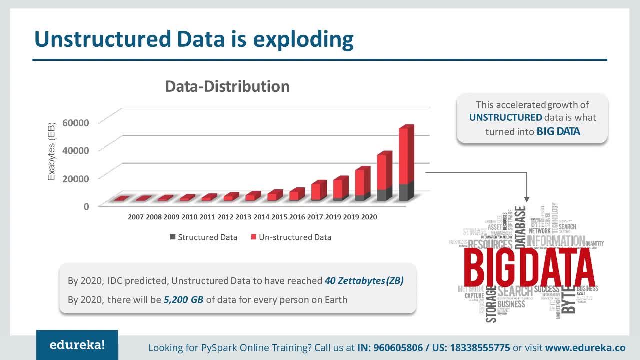 of those formats in one or the other Python lab. Python libraries also help you. support dealing with text that I have: mathematical formulae. You can imagine reading a white paper that has some description in the form of a text and then you have a complex formula, again some analysis, again a visualization. 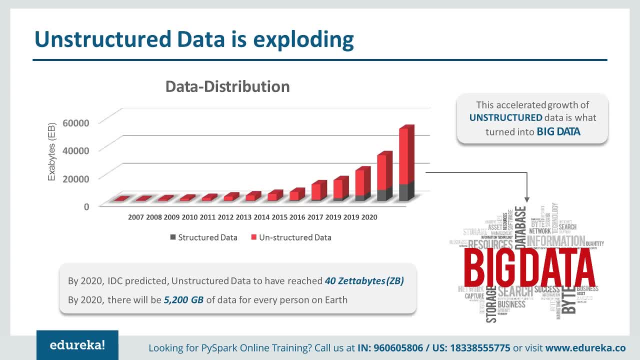 or a table supported with a complex form. Now, if you were to automate some of the understanding from these white papers, right, You will require a library that is able to understand or make some sense on whether the formula is related to a partial derivative or integral calculus. 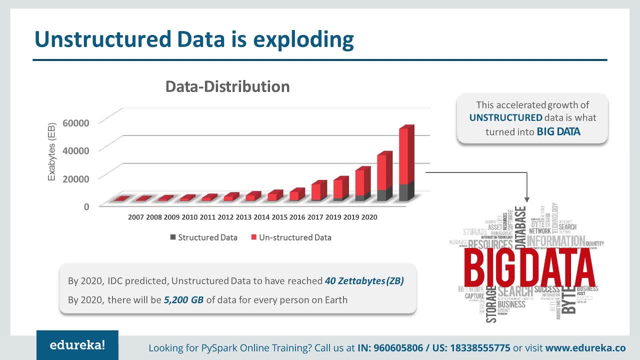 or does it deal with gradient descent in machine learning? So python has libraries to deal with those kind of formula understanding as well. Now that we know there are different complex formats of data, especially the last one that we are dealing with these days is not only complex. 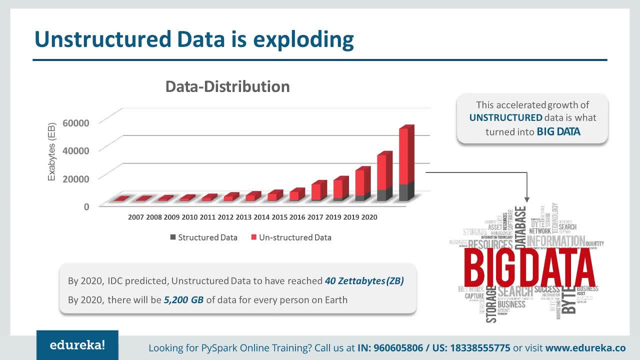 but it also comes in huge volumes when we say that we have the capability to process data in every format, and we do have big data these days to deal with any kind of volumes. So combine big data with libraries that can deal with any format and probably you are able to solve 99%. 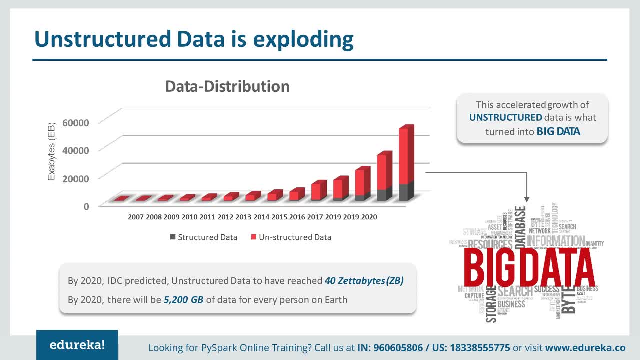 of the problem. So here are some stats on what volumes of data we can see by 2020.. So the data comes are predicted that unstructured data will likely reach 40 zettabytes- So zettabytes is over petabytes You can imagine- and by 2020 there will be 5200 gigs. 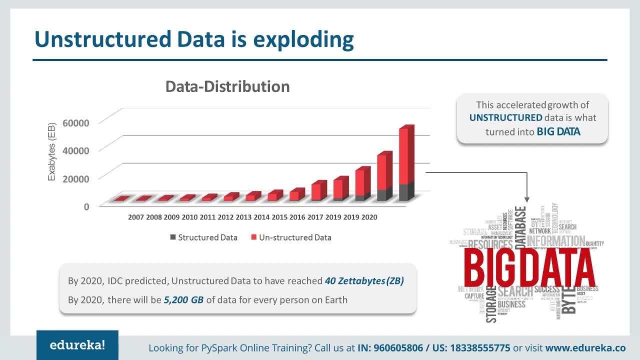 of data for every person on at least 5.2 terabytes for each and every one of us, and we are in 2018.. That's about it, And so probably another one and a half or two years that we are going to see this volumes. 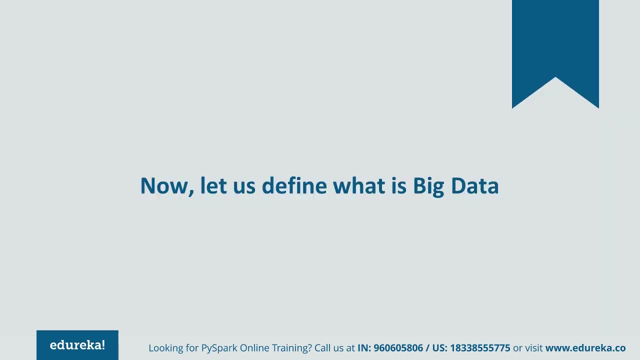 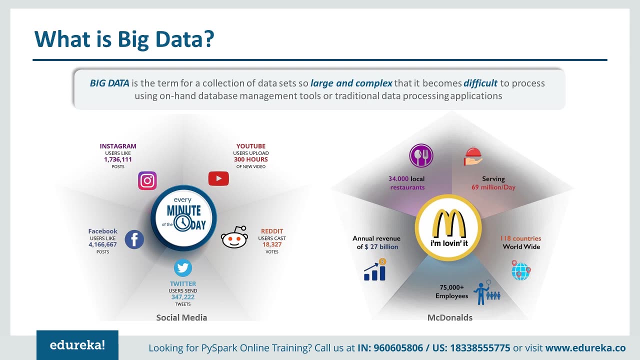 with everyone, and dealing with this volume is not going to be easy for any organization. They have to have big data appliances set up to deal with these volume. So even if an organization that is left out of this big data revolution, they have no choice. 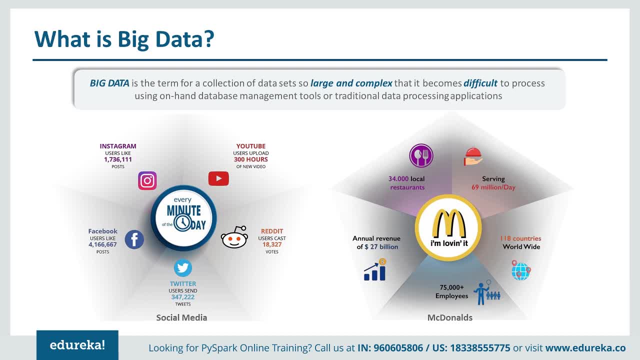 than to switch to it sometime in near future. So what exactly is big data? Does it go only by the name? that it contains big data? data that is really very big, big in the form of files or big in the form of volumes, So let's go through the term. 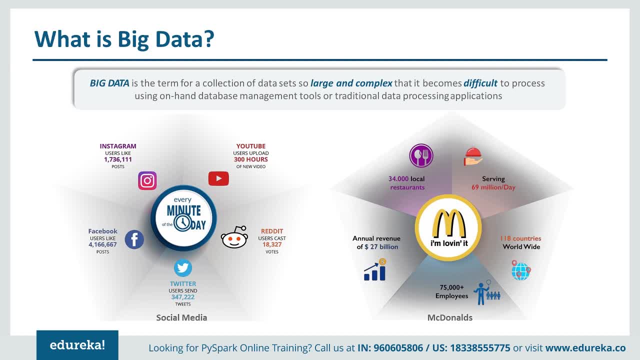 and understand some of the related examples that elaborate on it. So big data is a term for collection of data sets that are so large and complex that it becomes difficult to process them using a database management tool or traditional data processing applications. Now there are several key terms in this definition. 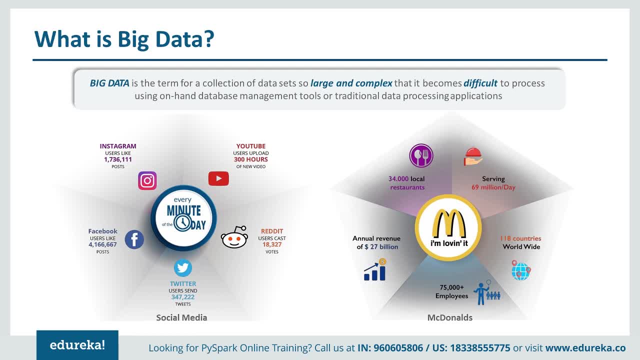 that we should pay attention to. first of all, the data is very voluminous and complex, and it need not always be complex. I mean, at times it could be simple as well, in the form of a CSV, but then the volumes could be significantly huge. 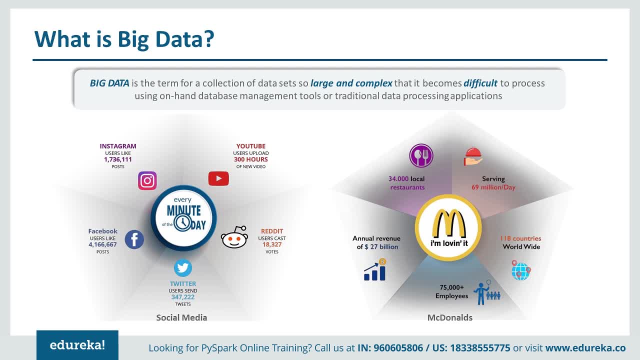 for you to. I mean that mandates them to be processed in big data. So the biggest benefit of big data is distributed computing. That means a task that can be performed by 20 person in one day will require one person to complete that task in 20 days. 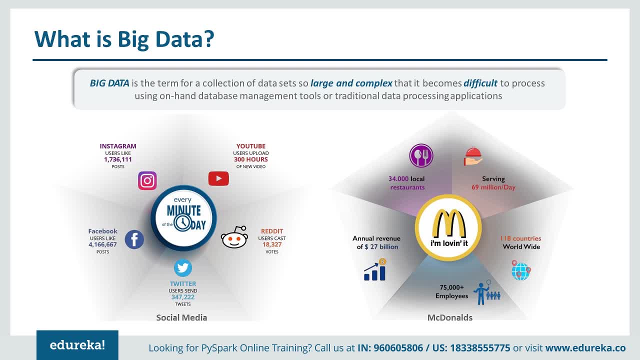 So the same analogy is drawn here, wherein if you have a single system processing that data, it might require certain number of days- and organizations cannot wait that much- for the analysis to be available, and on top of that there will be a lot of complexity. 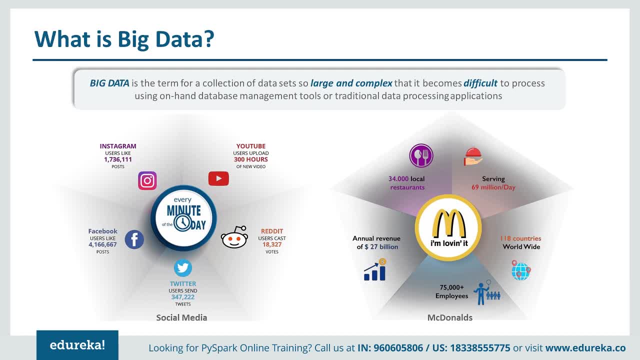 There will be a lot of failures in the process. If you do it batch by batch, you'll have to keep track of data And that does not mean the reader that you are processing. That's the final set. If you have such a huge volume. 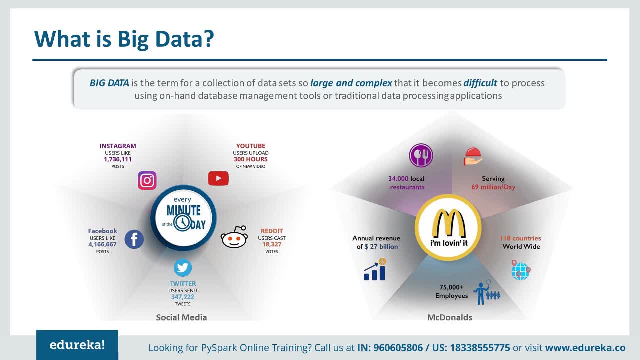 then they will be some mechanism generating new data every day. So while you catch up with the historical data, you would already have a huge pile up to deal with if you are doing everything on a single system, as opposed to that if you have an on-premise cloud. 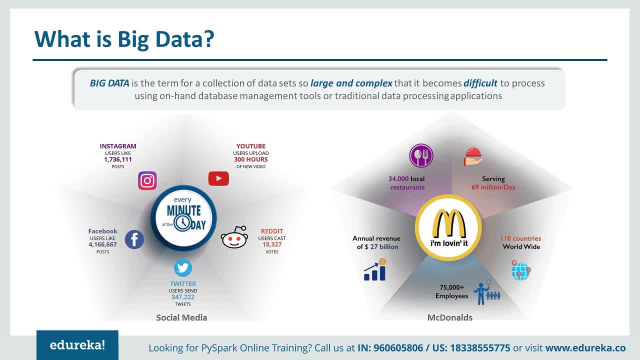 and on-premise cluster, or a public or a private cloud wherein you could set up a big cluster involving hundred machines with very powerful configuration, Let's say the four cores each 10 or 12 gigs of RAM in every system. right, It will involve cost, for sure. 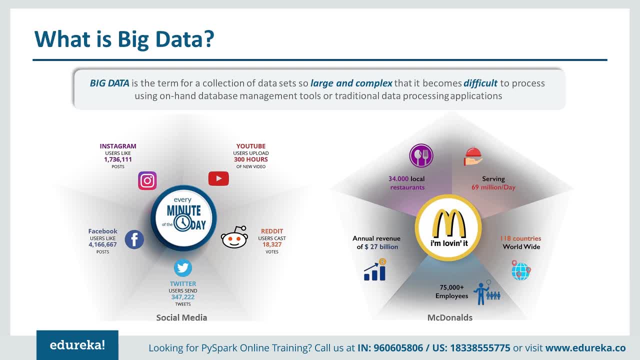 But then businesses know that the benefit of being in business lies in real-time data analytics, right. So they know that they are going to derive maximum value from this cost by getting real-time analytics out of that data, and that essentially means keeping the cost aside. 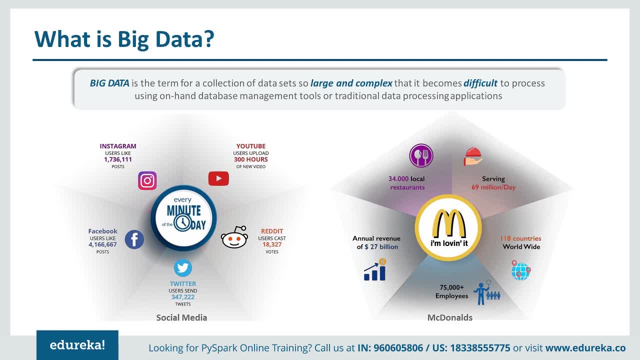 The analysis should be performed as and when data as seen by the system. That means there should be no lags, There should be no weights, and as and when data starts to grow as well, The cluster should have the property to also adapt to those increasing volumes to avoid any lags. 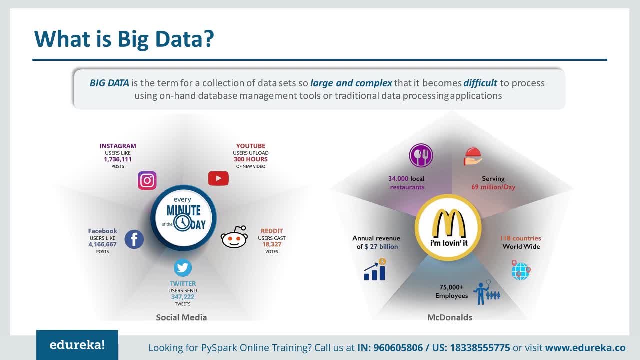 So some of the organizations that have already been some of the popular ones. I will say that I've already been using big data for quite a long time. We all visit McDonald's. even if we do not these days, we would have visited sometime in the past. 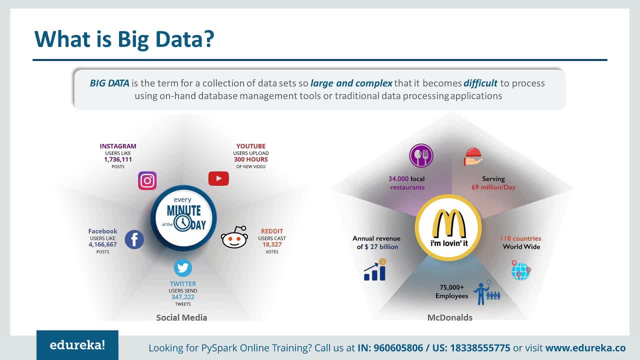 So McDonald's has huge volumes of data: It has 69 million burgers sold every day, It is serving in 118 countries 75,000 employees and annual revenue of 27 billion dollars. and, with respect to restaurants, They have 34,000 local restaurants. 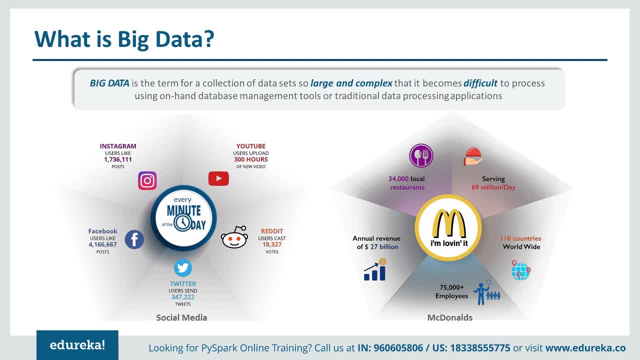 Now, if you imagine what kind of data it might be generating. So, first of all, you will definitely think of the transactional data. right, The burger sold, the price of the burgers, the revenue generated- Well, that's the core business data. 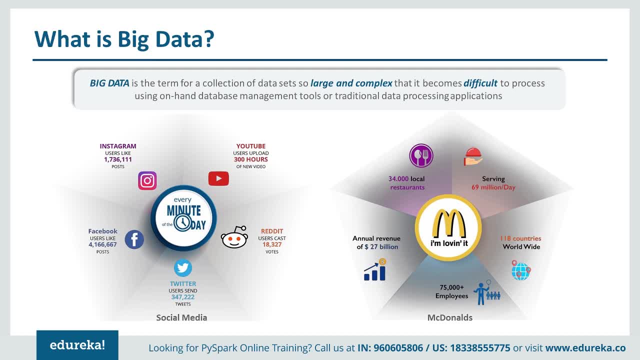 In addition to that, there will be data pertaining to employees, their salaries, their incentives, their issues, customer reports, customer complaints, restaurants closing up, restaurants opening up in new countries, new cities. How to keep track of all of this and how to come up with a system that is able to deal with all these changes. 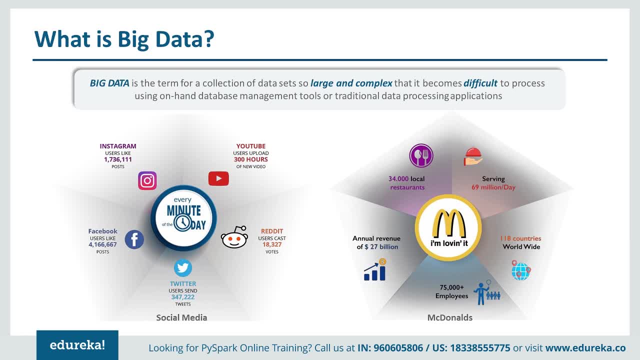 So they use big data for all this. and then, in addition to this, brands Like McDonald's or tell HP Apple, They are all sensitive on social media websites as well, to make sure if there is anything that is uploaded by a user that has the potential to become viral. 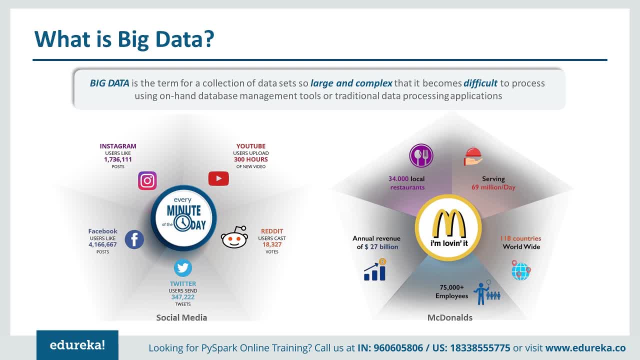 and affect their brand. They try to douse the fire as and when such a thing is noticed. So for that they have to constantly stream data from some of the popular websites that you already see here. But this is not the final list. This list keeps on growing every day with the addition. 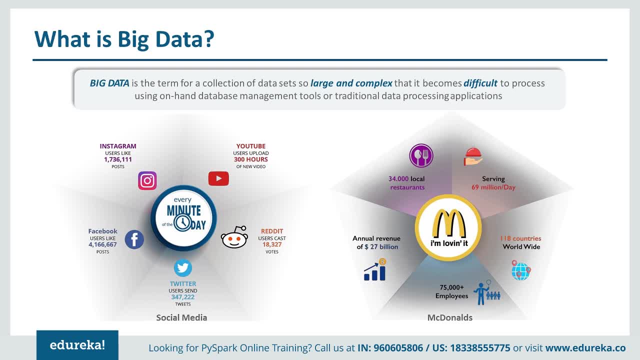 of new websites and social media portals. So you would have recently noticed, I think, Google plus closed its services. prior to that there was or code, and now we have Facebook, Twitter. nothing on the Google side, then. even LinkedIn is used by people for social media professional interactions these days. 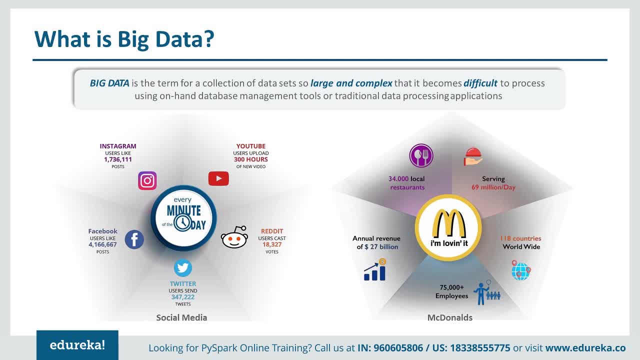 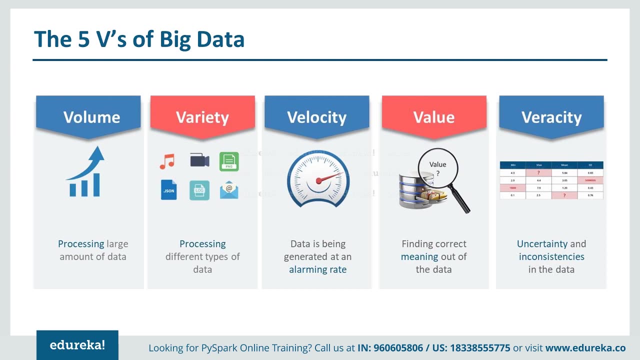 So organizations have to stream content from multiple websites and you can imagine what the volumes you would notice from these websites every day. It's humongous, definitely reaching over few terabytes. So now dealing with all these different problems, right? How does big data address so much of complexity in data? 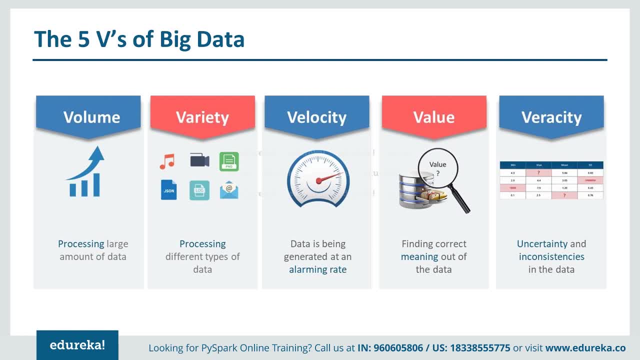 and high volumes and data. that's largely because of few of the properties that big data has inbuilt, and all these properties start with letter V, So we say the five V's of big data. and, to begin with, big data has the ability to deal with huge volumes. 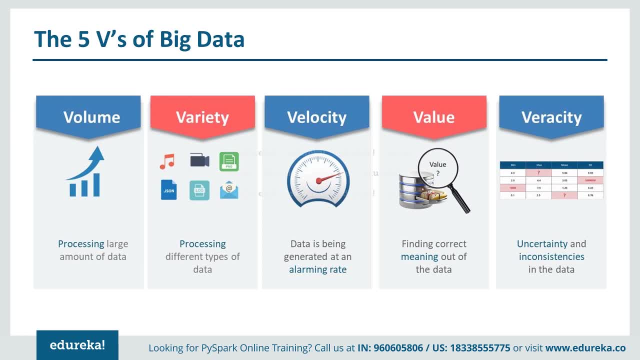 You can process variety of data in big data using any language you want to use Java, You could use that. you want to use a mix of Java, Python and Scala. You can have pipelines defined in with some of the jobs written in each of these languages or in a combination. 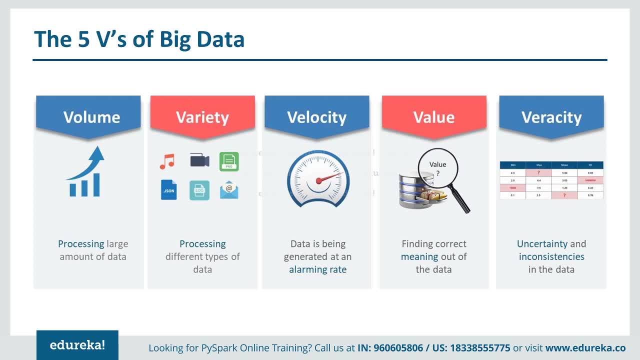 of these languages, So that will give you a flexibility in dealing with any kind of data format. velocity Data is being generated at an alarming rate in every industry, in every appliance, in every solution. So no industry is an exception in this case. So big data is able to deal with the rising volumes. 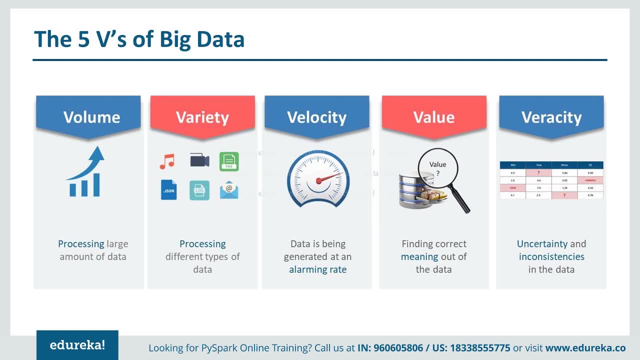 and data. It is able to find the correct value out of the data. So if you want to do analytics, if you just want to aggregate data, it will be able to do that. If you want to transform the data, you'll be able to do that. 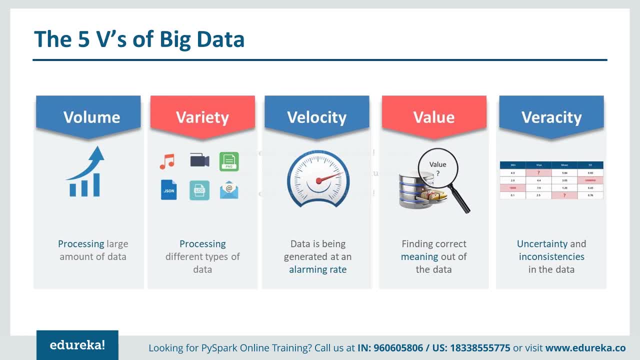 If you want to prepare data so that it can be fed to a machine learning problem, You could do that in big data, and running machine learning problems is not that easy because, if some of you are already familiar with the process, it involves training a model on a data and then using that model. 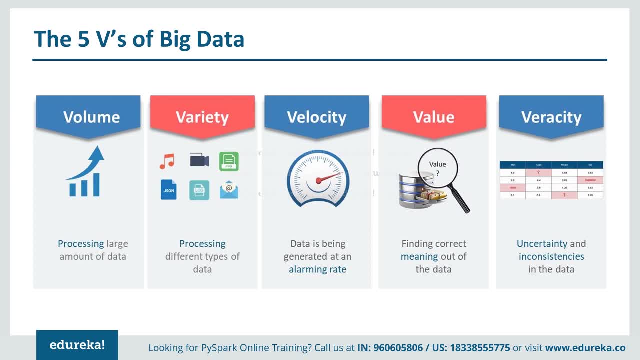 So what if you say that you want to retrain your model every three months so that it is able to give you better insights based on its learning, on your data set as well, right Now? if you say that the data is coming in numbers of terabytes every day, and if you're talking on a scaling? 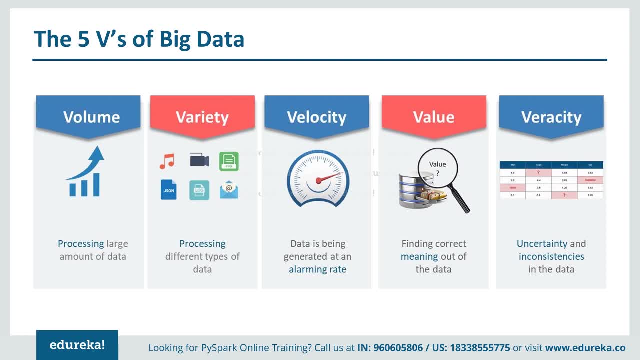 the model on or retraining it every six months. so it will be 180 terabytes in last six months, assuming you get at least a terabyte a day. So minimum of 180 terabytes, and in addition to that we are also taking into consideration the historical data. 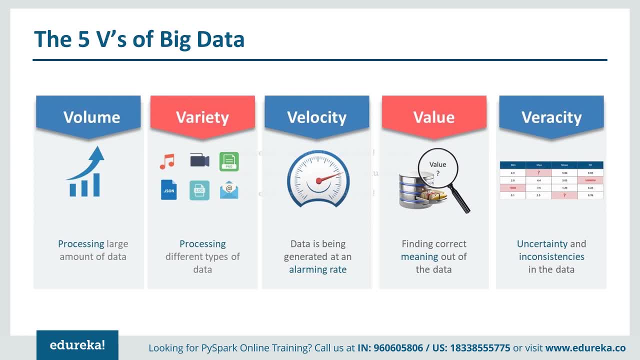 So big data supports all of this to be performed in a big data appliance using machine learning libraries, and we will see some of the tricks in modulate when we touch upon machine learning hands-on. and last is veracity, wherein often there is a doubt in the mind. 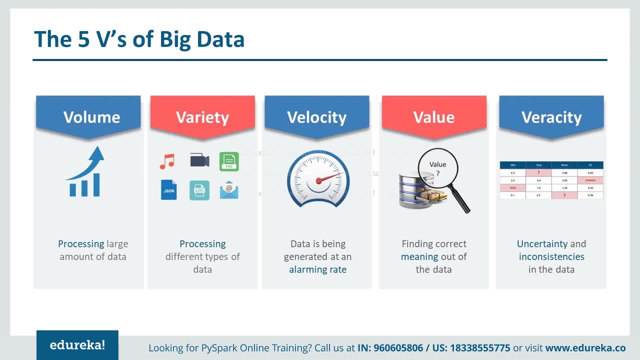 of companies who start using big data. You are getting results, But at times, you will see, the results might not match some of the conventional reports that were drawn from a relational rdbms right. But then there could be several reasons for that. one is: 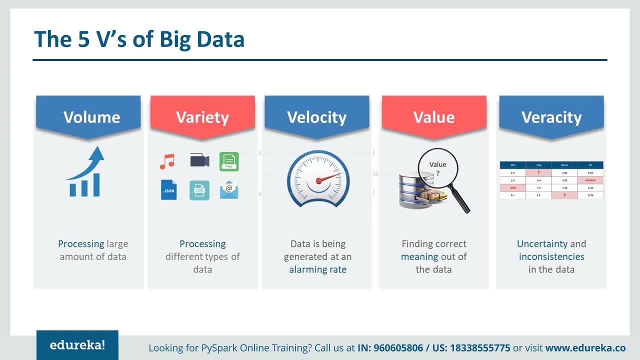 probably as part of the migration, something would have been missed from rdbms to a big data transition, or they could be something lacking in the current process or in the legacy process, Due to which you see such a discrepancy, but then the certainty, uncertainties in the results often. 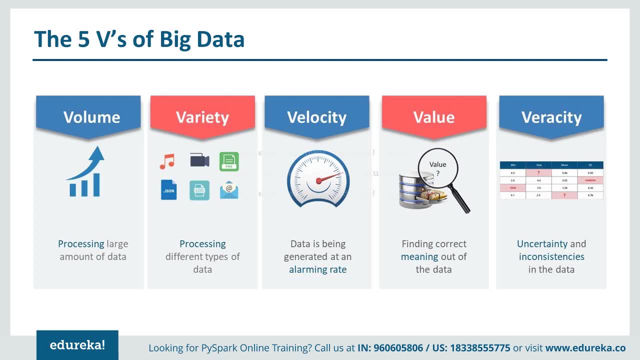 lead to conclusion that probably something is wrong with the new thing that I have migrated to and that cast a doubt. so that requires some kind of checks and data quality to be implemented in every big data appliance to make sure that you are not losing a single record. 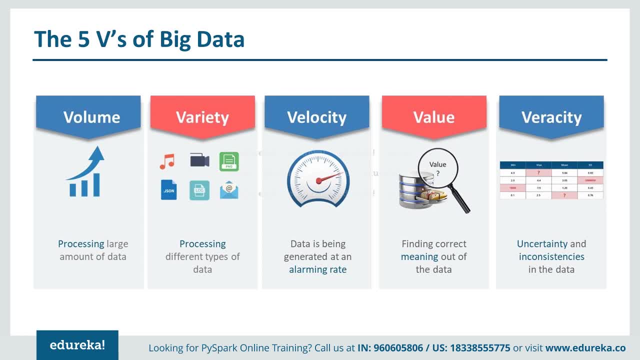 as part of the process. It could be due to some of the fallacies in the process established by a developer as well, So the fault could be on any side. but then, because of these five promising attributes of big data, it is the preferred tool for processing data these days. 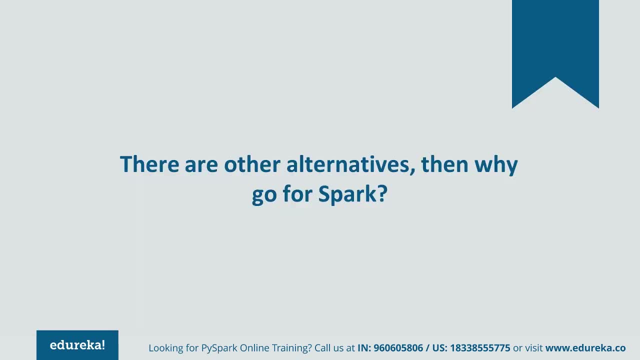 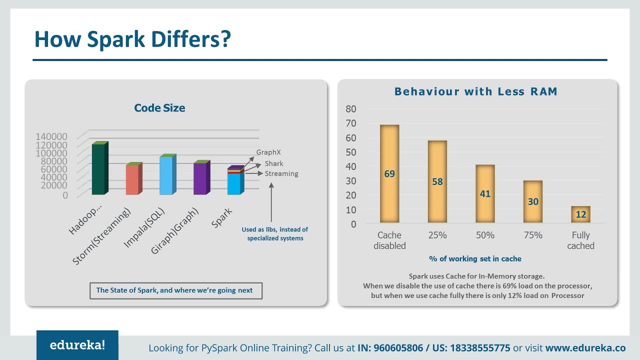 With respect to the two types of processing that we discussed, There are several alternatives, but then why is this park often considered as the preferred alternative? So here are some of the stats that bring out the capabilities of a spark. So, when you look at the code, 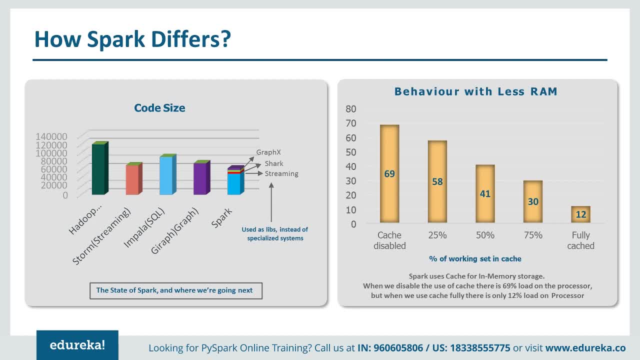 size. often it is believed that the lesser code you have to write. lesser is the maintenance and lesser is a debugging effort. and that is why Python is preferred over the languages these days, because what you would accomplish in Java or C++, writing several lines of code, might be accomplished. 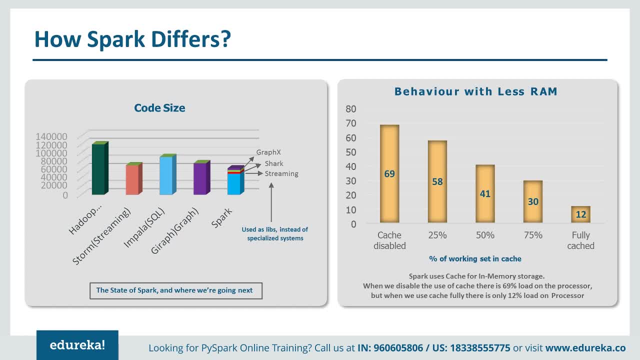 in a single line in Python, Similarly in a spark, as compared to Hadoop, wherein you would write 140,000 lines of code, The same could be written in around 60,000 or 70,000 lines in his park. So almost half of that storm streaming again has lesser amount. 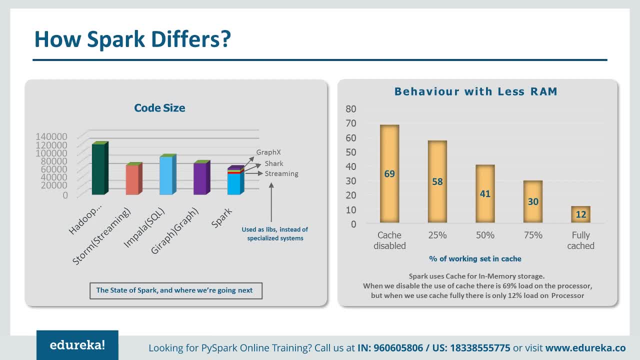 of code to write, but that has its own set of limitations. Impala has certain number, giraffe, or the often referred as graph, that again has certain lines of code to be written. but a spark supports graph, It supports SQL analytics, It supports streaming and the amount of code that you have. 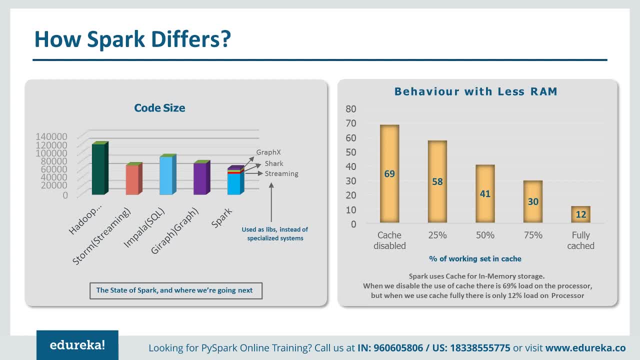 to write all put together will not exceed even the half of all the previous four put together, So code size is often very less when it comes to writing the same thing in a spark. on top of that, the performance of a spark is pretty good as it processes everything in the memory. 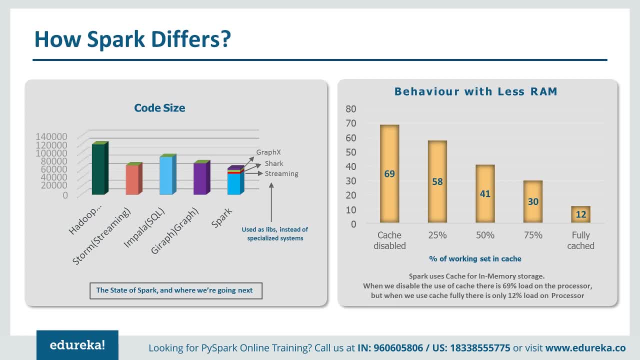 So when you have to check on the behavior of any of the applications that you set up, in terms of the output of those applications, so their behavior can be compared over the usage of the RAM. So if the cache is disabled, a spark will actually take 69%. 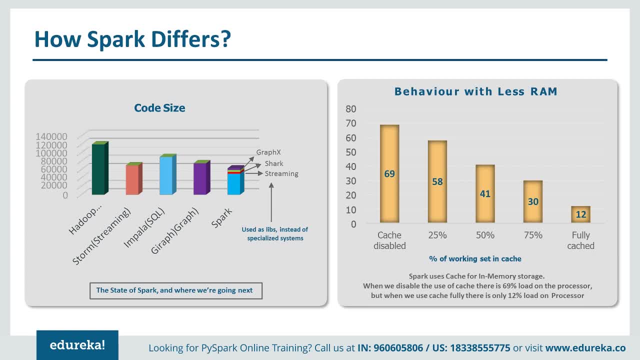 of the memory if it is enabled to an extent of the memory. If the cache is of 25%, it will take 50, but if the operations are fully cached in a spark, it will only take 12% of the time required to process. 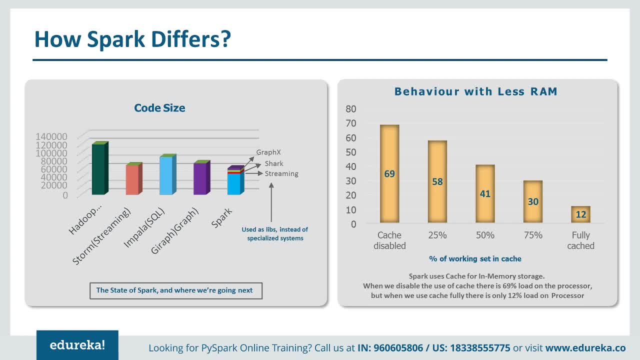 the data that would otherwise have taken eight times of the actual time. So 12 into 8 will make it hundred percent. So spark uses cache for in-memory storage and when that is disabled there is 69% load on the processor. So Hadoop does not have this cache behavior. 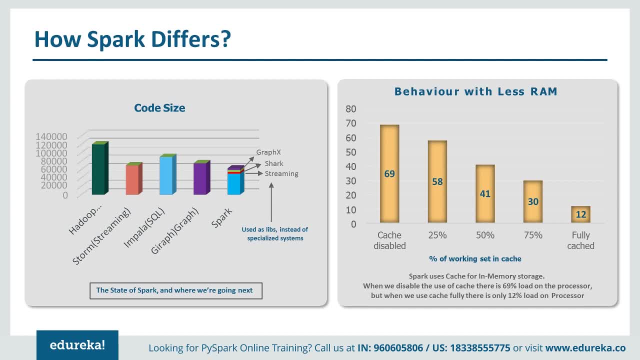 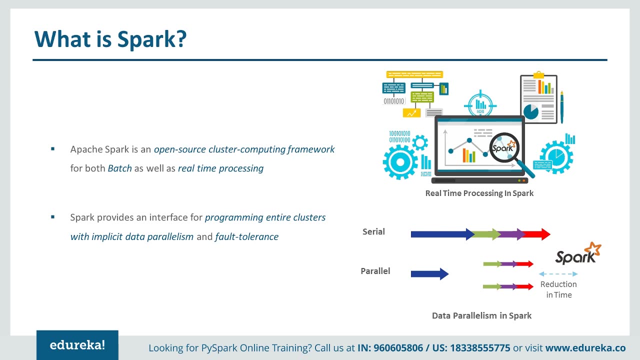 That means if you run a spark without any caching, it's equivalent to doing a Hadoop kind of operation, and that essentially means it will take almost six times the time as taken by a fully cached spark application. So, having said, talked about compelling reasons for choosing a spark over other appliances, 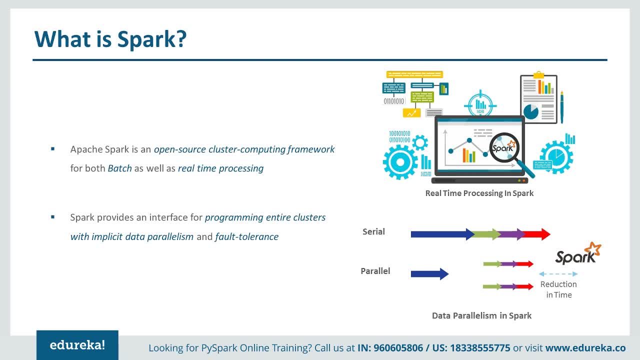 We should also know what exactly spark is. So first of all, it's open source. You don't have to pay a penny to use a spark. You can try it in a clustered mode on cloud or on-prem. You can try it locally, setting it up on your laptop. 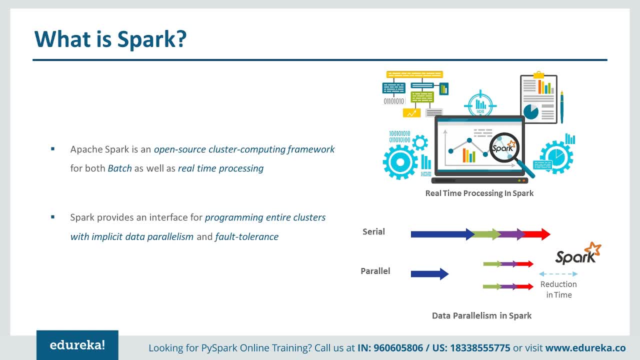 You can try it on a docker, You can try it on kubernetes on your laptop. So there are multiple ways in which this can be set up, which might not be possible with any data warehouse. You cannot set up data warehouse on a local for testing. 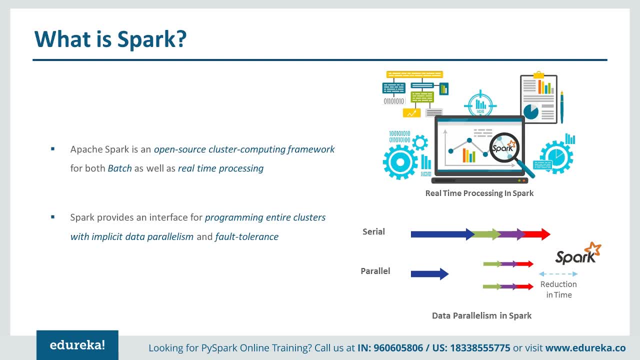 So it is open source. It is a cluster computing framework, So everything works in a distributed mode wherein you can specify- you also have the ability to specify how many processes you want to tag to your application from a distribution perspective, What kind of memory you want to make available for your process. 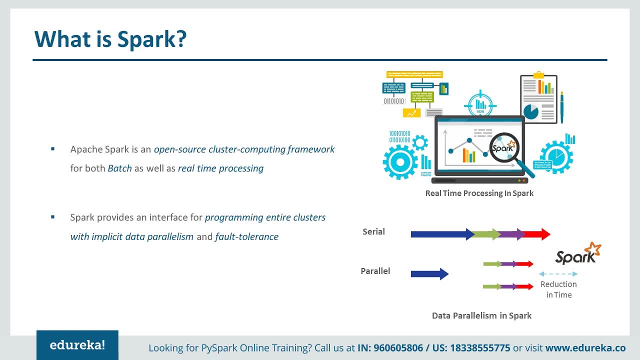 So all that is possible when using a spark. you can run it in his batch or in a streaming mode. batch often will involve dealing with historical data and the streaming mode will involve dealing with real-time data that keeps flowing in. it also provides an interface for programming entire clusters. 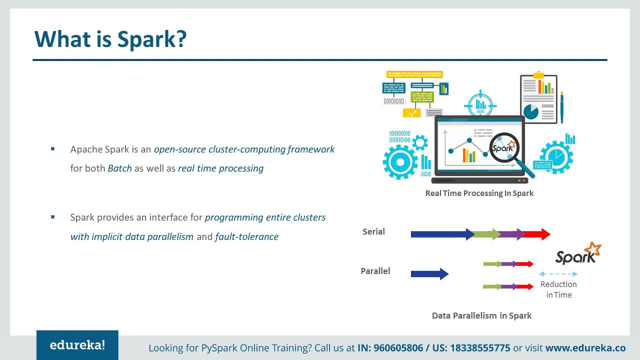 with implicit data parallelism and fault tolerance. So when we say it provides an interface, we don't have to implement these properties in our scripts, which otherwise were required in when writing map reduce to an extent. So when MapReduce programs were written in Hadoop every stage. 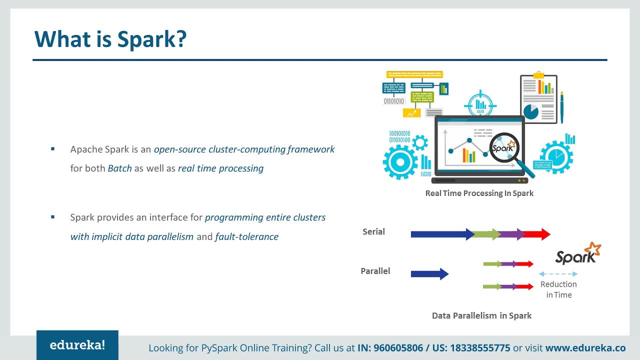 has to write its output back to HDFS as an intermediary output for next stage to pick that up and process. but a spark deals with that very elegantly. We don't have to write those intermediary outputs because it does everything in the form of a lazy evaluation. 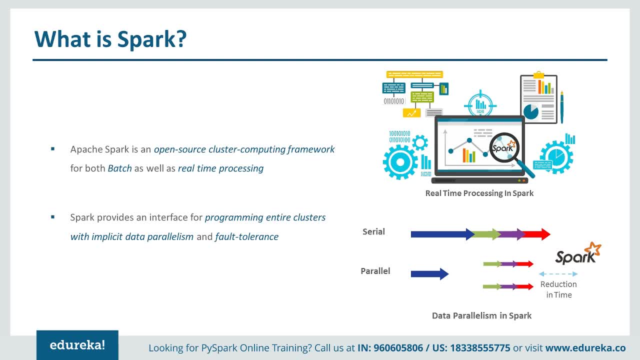 Secondly, a spark does all processing in memory. It does not have to be taken off the memory, written to disk and then again loaded into memory. It's there in the memory. So all of the processes run at once on the same data set. data parallelism and fault tolerance implicitly implemented. 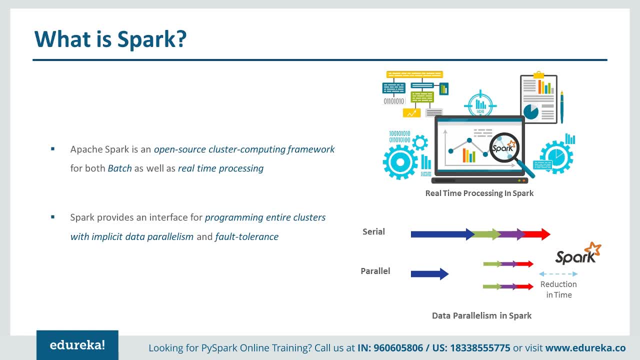 in the interface that is exposed by spark. So the basic interface that a spark exposes for programming is the resilient, distributed data sets. These are the kind of basic objects that we deal with in a spark and they already have these properties embedded. So when you submit an, a process, 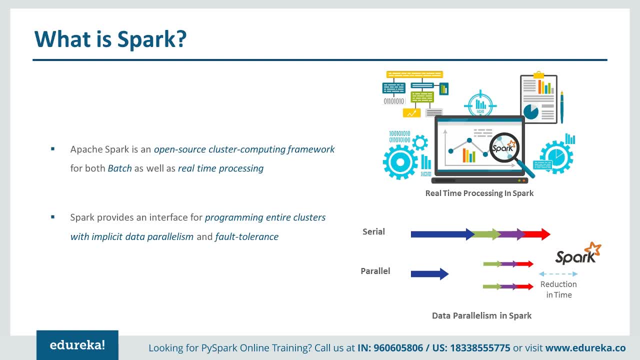 or a job to run using these objects. it will automatically run on multiple machines, making use of Ram distributed over multiple machines. It will take care of fault tolerance as well, and it will do speculative processing as well, Wherein, if it identifies any process that is running slow, 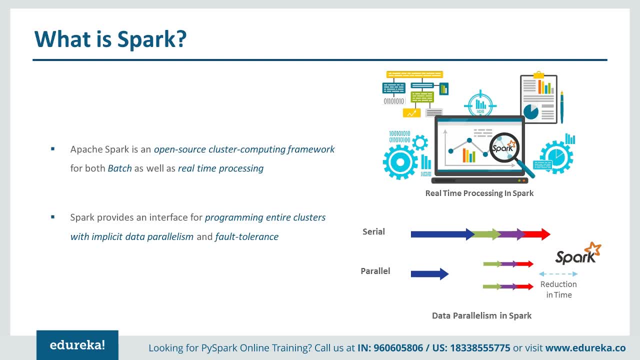 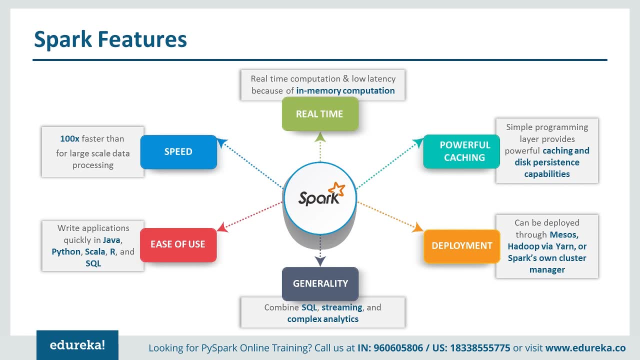 It tries to rerun the process on its own, without us giving it an indication that it should restart something, while spark has all those capabilities in addition to that, These are some of the features that really make it a very powerful application to learn. first of all, 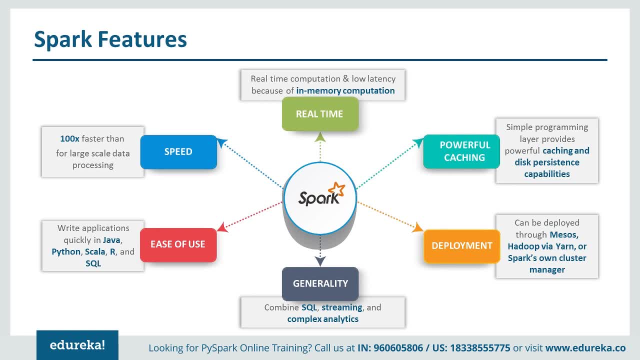 it has the ability to do real-time computation, which was lacking in earlier versions of big data processing frameworks. So it can do real-time computation and it has low latency because of in-memory computation. latency always pertains to transfer of data between memory and hard disk and back. 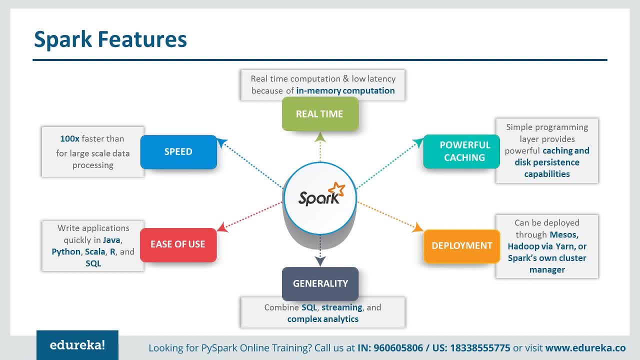 So if that is not required and everything is in memory, the time is saved to a significant extent. It has powerful caching features, So simple programming layer provides powerful caching and disk persistence capabilities. We can run our programs by default in memory. In addition to that, we can explicitly cache objects. 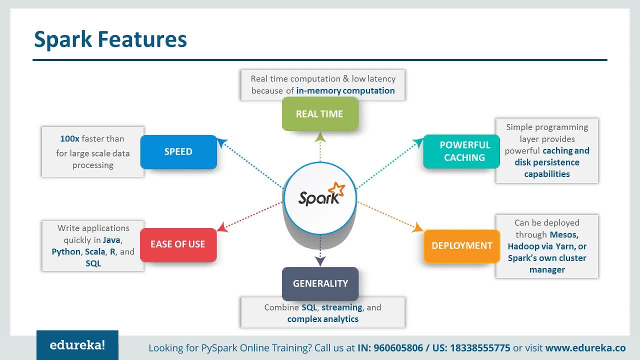 We can explicitly uncache objects or deeper system. We can also choose if, at any point in time, we want to save something on disk. So it provides that interface to us through which we can do either caching or save something on disk directly. then, when it comes to deploying a spark, spark can run. 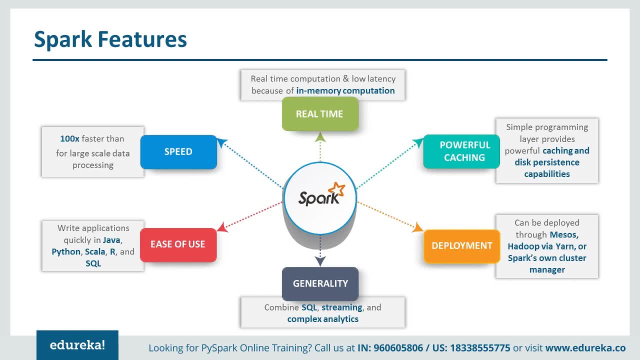 on its own without any external tools. First of all so it has its own cluster manager that keeps a track of all the components in the cluster and all the jobs running on that cluster, which we refer as applications in this part. but it also has support of integration with mesos and yarn. 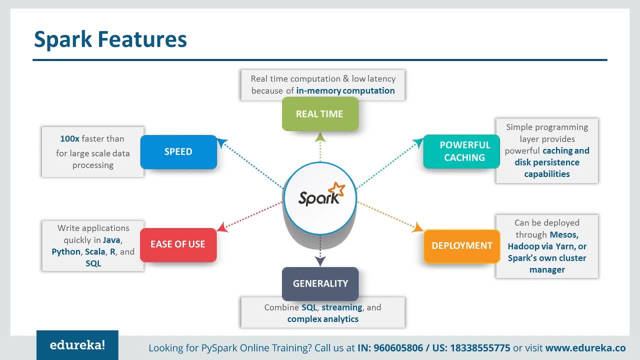 So, in fact, in a spark version to yarn is the default resource manager that comes along and we will touch upon yarn as well. So it is a very good resource management service that takes care of allocating resources to any of the applications that we wish to run. now, when it comes to data processing- all 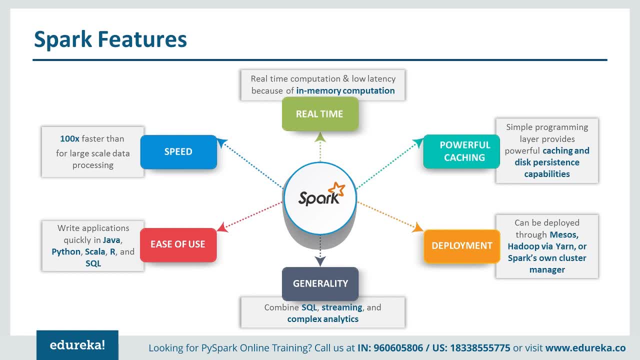 of us come from different background. Some of you might be very good in Java programming or any kind of coding that you have been pursuing in last couple of years. Some of you might be very good in sequel and some of you might have extremely good capabilities. 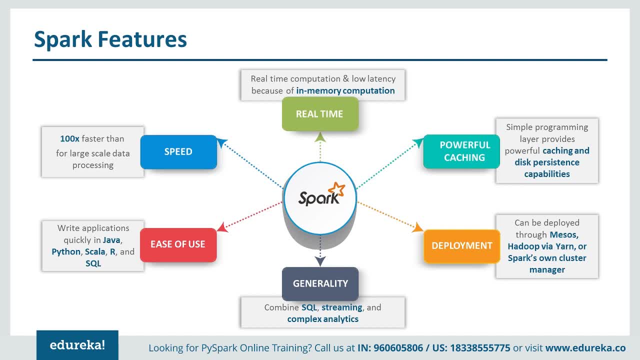 in terms of analyzing data in the form of pandas data frame in python or an equivalent kind of data frame in our now is. power gives us the ability, first of all, to use different Languages to connect with a spark. It could be Java, python, Scala, R and sequel. 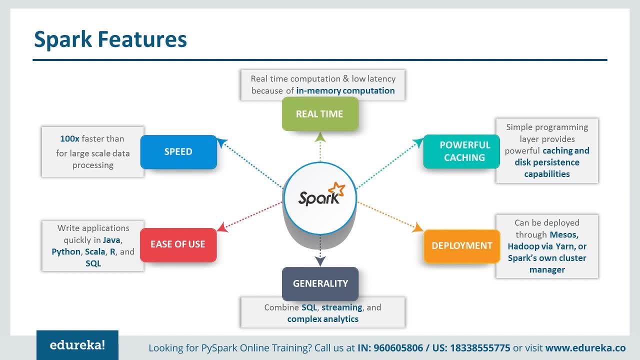 That's ease of use. secondly, in addition to that, We can also decide- how is it that we want to analyze data, whether we want to analyze data using sequel, whether we want to analyze data writing a bunch of spark scripts involving the use of streaming module. 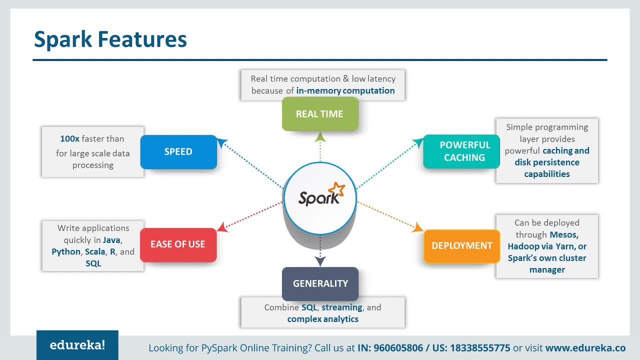 or we want to do complex analytics using machine learning. that involves some familiarity with those concepts in Python, So it supports all of that. So if you are coming from any of these backgrounds, you do find some level of comfort in one or the other module when it comes to analyzing the data. 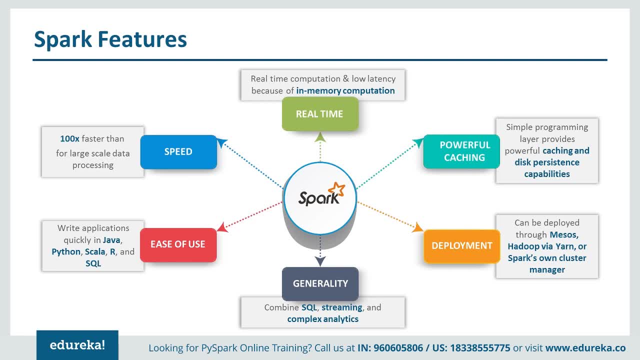 Lastly, where did big data start and why was this actually required? So, right from day one, the onus of using big data for any kind of process, first of all, is to have a real-time processing and second is speed. So, as I mentioned, if you have data showing up in your system, 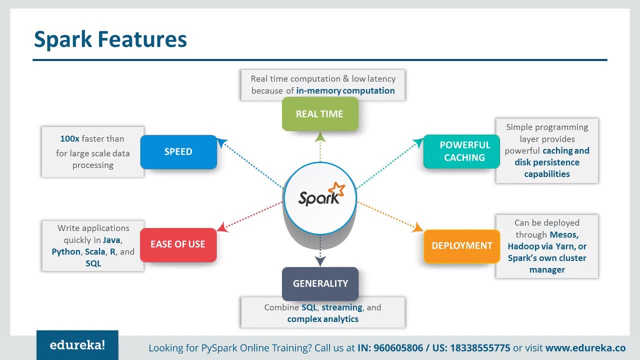 Now you want the results also, or you want it to reflect in your reports now, and this now is tolerable up to few seconds or few minutes, but not beyond that if you are running a big data. So speed has always been an important factor or important driver for taking everyone to big data. 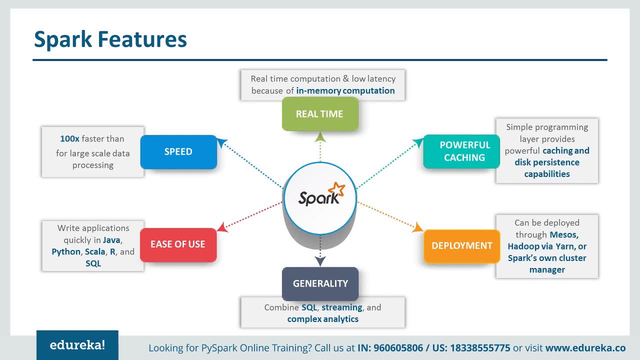 or it is hundred times faster than any of the conventional big data appliances for large-scale data processing. This is proven. you can Google this and you will find millions of examples wherein people have set up notebooks and examples to show how a spark runs hundred times faster than Hadoop. 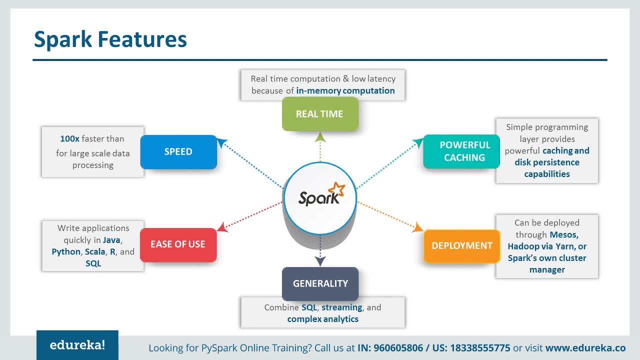 So chakrapani, sequel again, is a kind of language. That is the reason we say sequel also comes in ease of use. So if you just know how to create a data frame in this part, so after running few lines of boilerplate code, 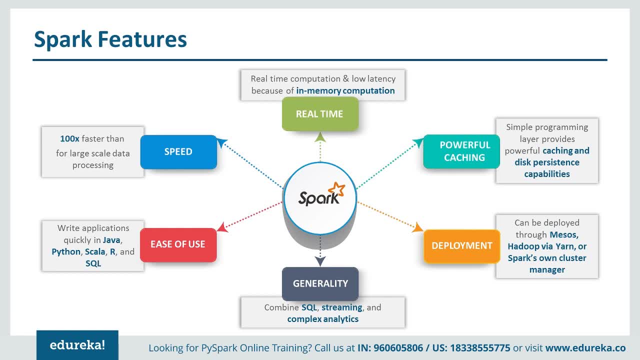 all you need to do is know how to write a sequel and how to run sequel on that data frame. So sequel again will stand out as a language and that's why it's included in the ease of use. but technically speaking, when you read the spark documentation, 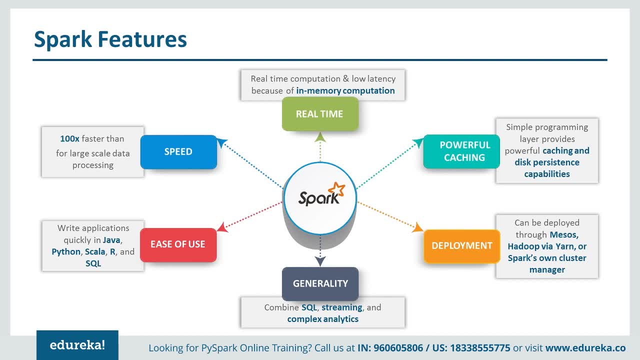 and you try to find out what languages are supported for integration. with a spark, It will only be Java, Python is call and R and it could be something else, but not sequel. So from that perspective sequel won't stand out. Let's move ahead and understand few domain scenarios, big data. 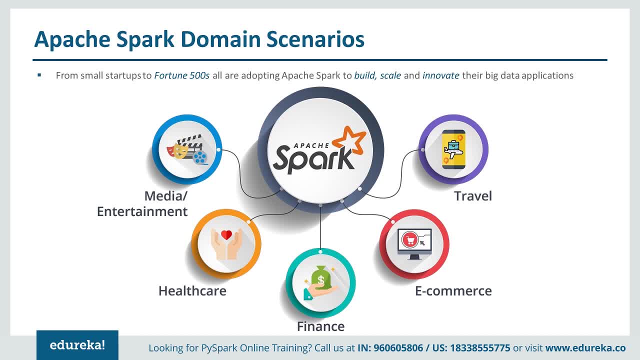 is using every domain these days that you can think of and it is not only a tool that fortune 500 scan afford because it's free and runs on cheap computing cluster wherein you can just plug few ordinary laptops and set up a spark on it. You can very well run a spark at your home. 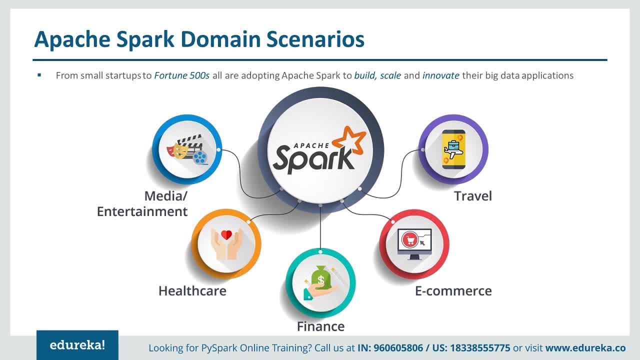 If you have few of such machines and you can run it on your laptop as well for testing and other development purposes. So all organizations are adopting a spark to build a scale, innovate their big data applications. You know, has a bunch of properties that are highly personalized to maximize relevance. 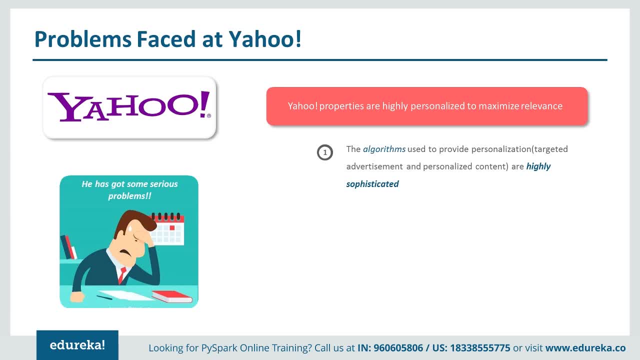 and the algorithms that are used to provide that personalization are again very sophisticated. They have targeted advertisement and personalized contents and delivered through these sophisticated algorithms. that model must be frequently updated to keep pace with the time. That means as and when new data keeps coming in the model. 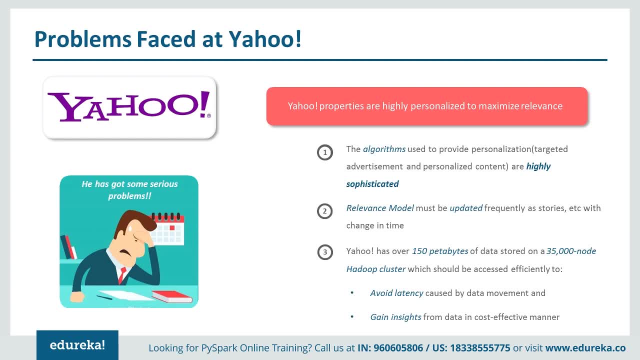 also has to update itself. So the challenge is: Yahoo has 150 petabytes of data stored on 35,000 node cluster and that needs to be accessed efficiently to avoid latency and gain insights, and that is why Yahoo choose spark to process all of that data. 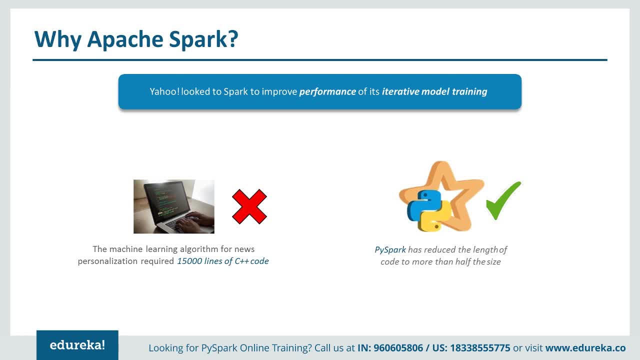 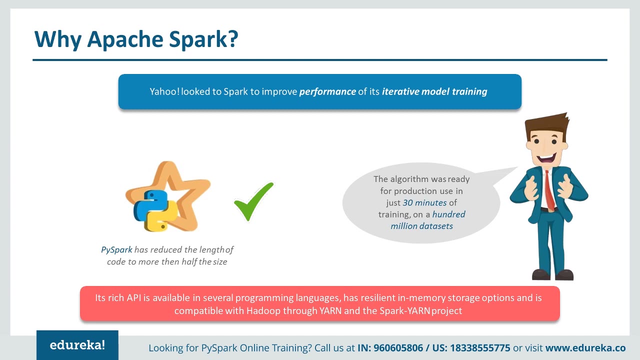 It had machine learning algorithm for news personalization and that had 15,000 lines of C++ code and pi. spark has reduced the length of code to more than half the size because, first of all, writing code in Python would have been simple and combining it with the spark paradigm. 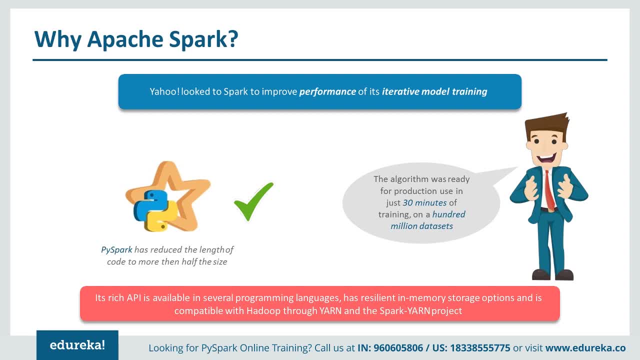 Secondly, it would have also made available some of the MLM algorithms and processes that otherwise would have been difficult to implement in C++. So Yahoo claimed that the algorithm was ready for production use in just 30 minutes of training. So to use the spark for personalizing its news pages. 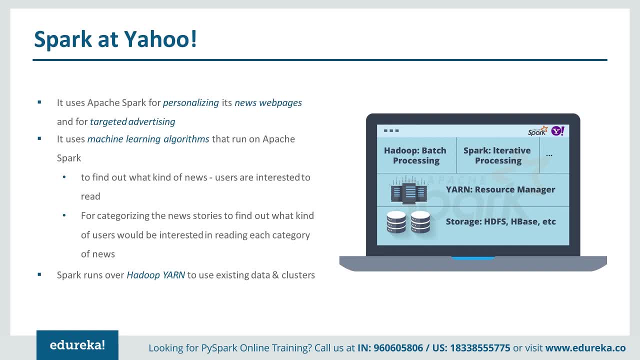 It used machine learning that runs on a spark to find out the kind of news the users were interested in for categorizing the news stories. all of that runs on Hadoop yarn to use existing data and clusters. So Hadoop was already there in place holding all of that data.